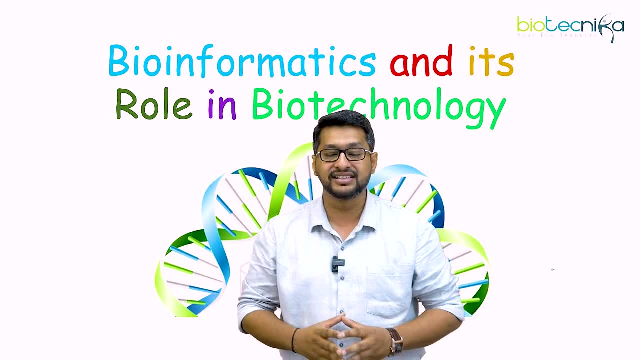 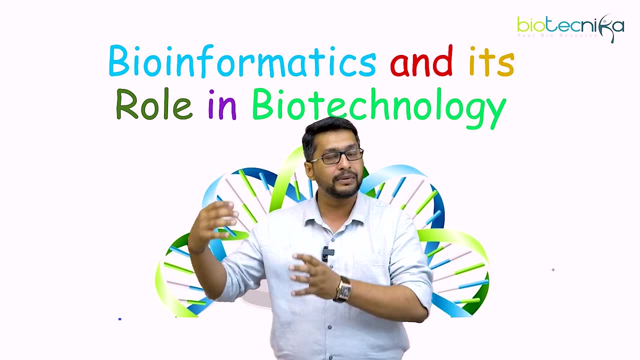 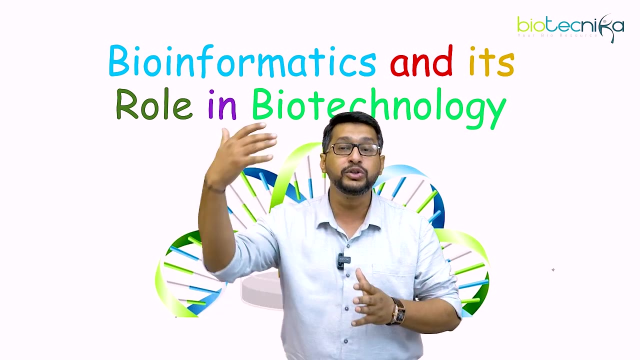 Now, before we start, we'll try to understand What exactly is biotechnology. Now, if you remember, bio and technology: bio refers to biology and technology refers to a process in which you can- you can actually maximize the efficacy and you can utilize the applicability of a particular technology onto biology. 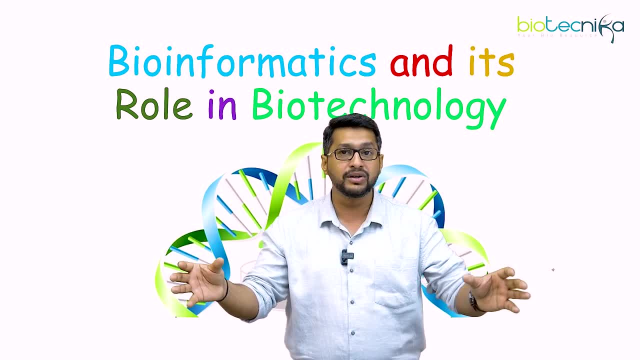 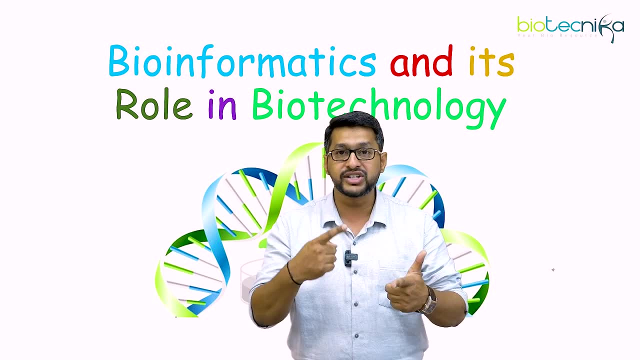 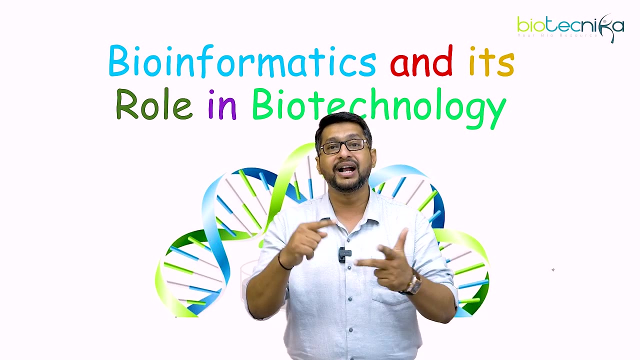 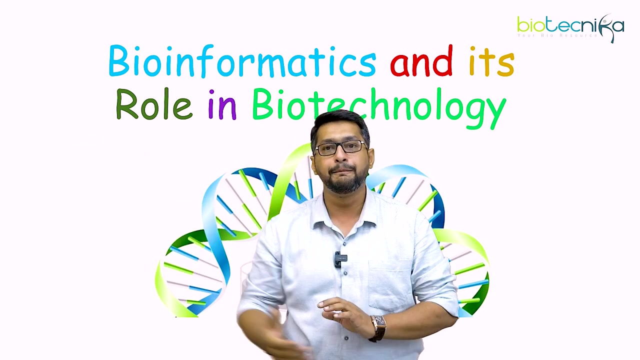 Now, why do you want to use technology with that of biology? This is to explore newer components, and newer components which can lead into better food, newer components which can lead into better food, Better pharmaceuticals and newer components which can lead into better cosmetics. So you know, food, pharma and cosmetics are the three important fields in which biotechnology has actually created a completed boom which has been actually seen from the last 10, 15 years now. 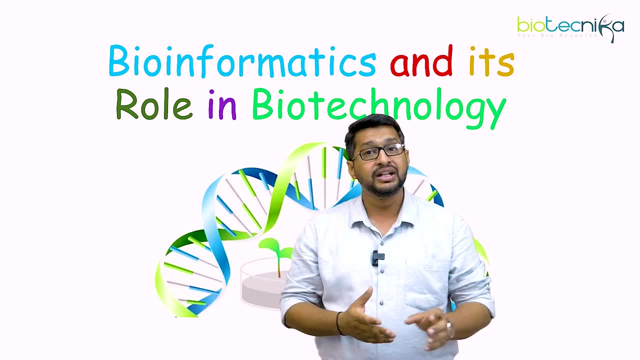 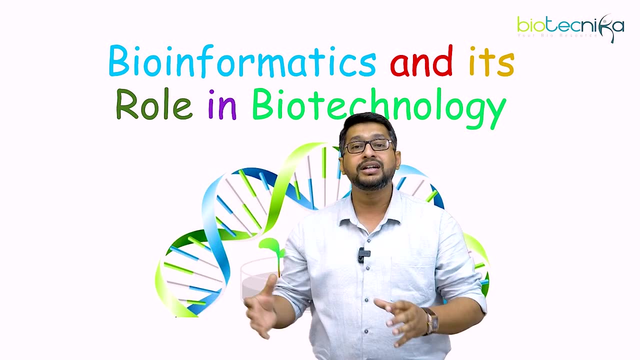 So this was with regard to biotechnology. Now, what is bioinformatics? Now the you know, the data, what we have got from biotechnology is so huge. It is so big that, you know, manually curating data becomes impossible for now, because of the huge data. 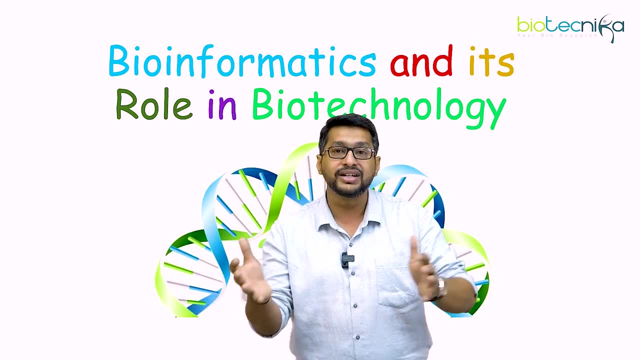 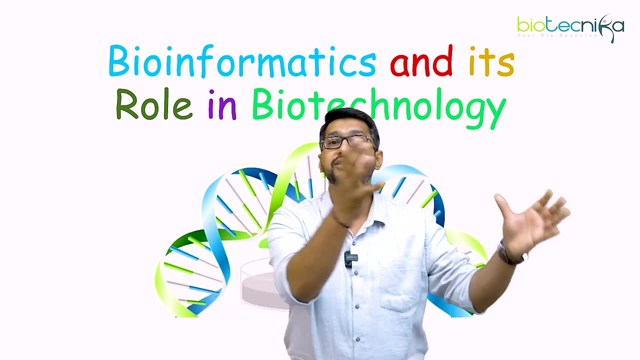 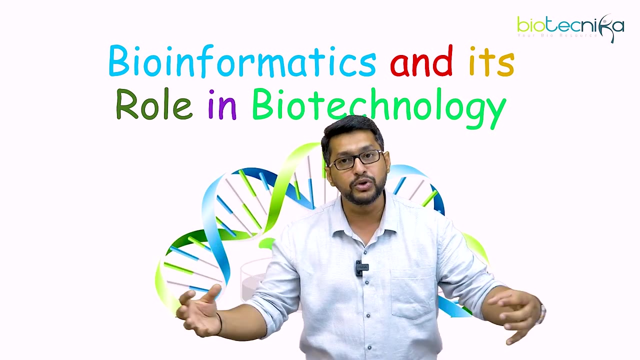 So what we need to do is we need to use technology to understand biology, and especially, this technology is computer science. Now I'm using the power of computer science to understand biology And if I am trying to amalgamate biology and its understanding with that of computers, this branch is called as bioinformatics. 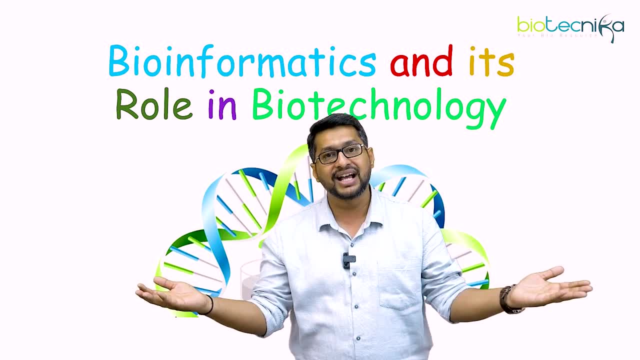 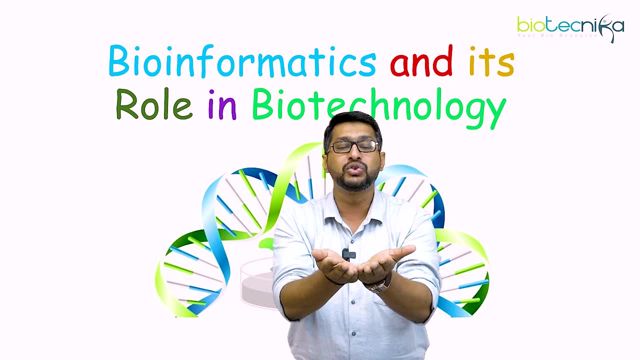 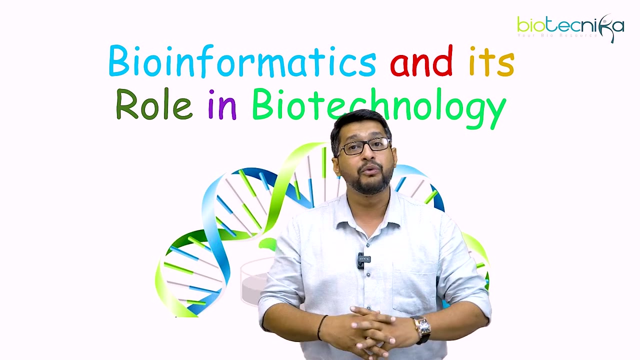 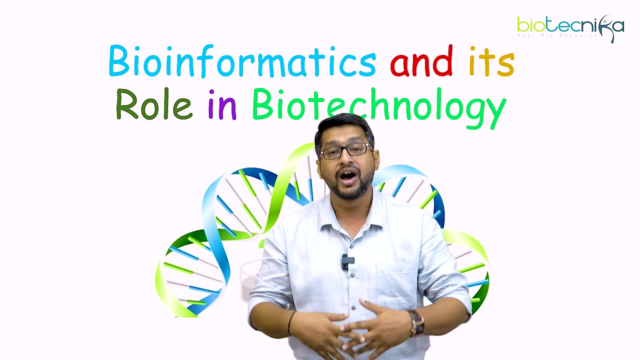 So now, at one hand, I have biotechnology And on the other hand, I have bioinformatics. Now let us try to see what happens when we have a marriage, when we amalgamate these two sciences, and this can lead into an entire newer science, and this science can actually help in understanding. you know, various kinds of you know, challenges, various kinds of opportunities which can actually be explored and exploited for the benefit of humankind. 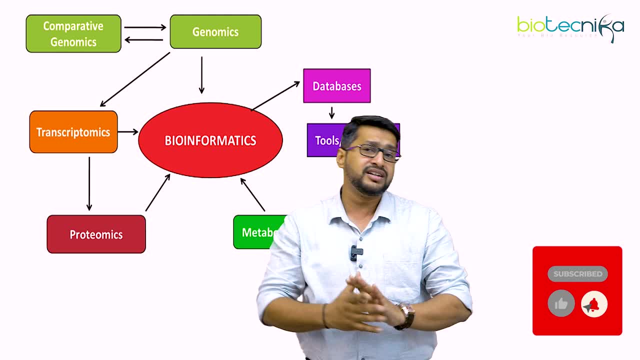 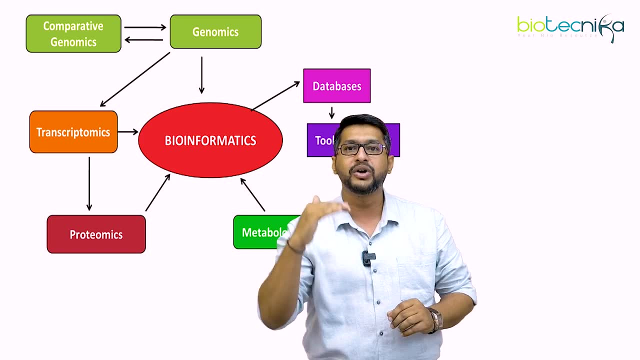 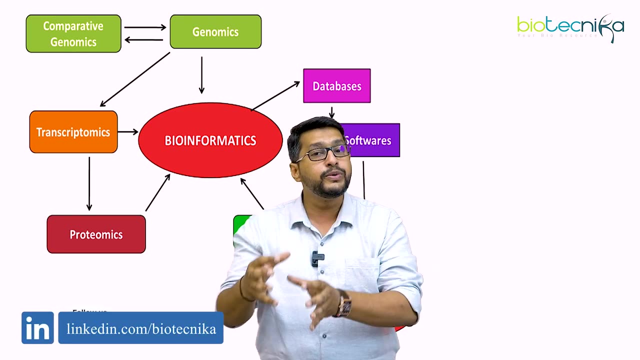 Now we start with central dogma. Now, when we start with central dogma, we know that it is Genomics. from genomics you have transcriptomics and from transcriptomics you have proteomics. But, however you know, the understanding of genomics was so vast then people thought: why don't we extend the component of genomics to an other level? 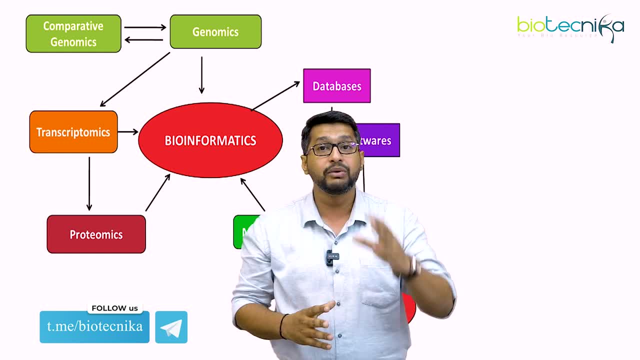 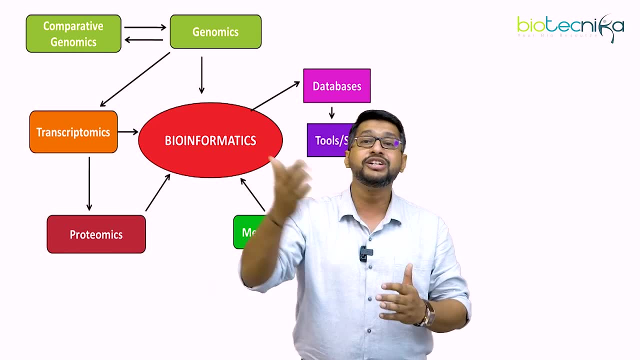 And this higher level is called as comparative genomics. Now, in comparative genomics I would compare between you know, host to pathogen interaction, host host interaction, pathogen, pathogen interaction, pathogen with biotic interactions and pathogen with. 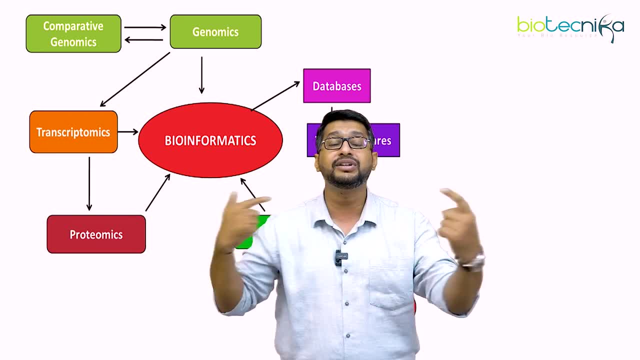 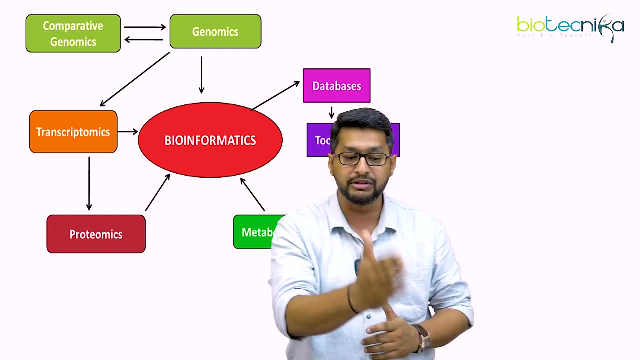 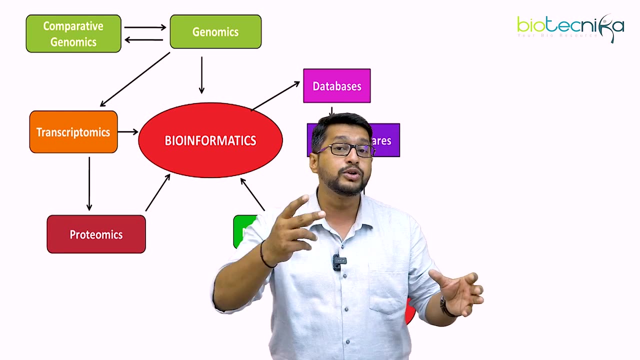 Biotic interaction, So I can look into the various components, so that I can have a 360 degree view of a particular genome. And that is very much, you know, which is possible with, you know, comparative genomics. Now this genomics could be again looked into its transcriptomic level, wherein I am looking into the gene expression pattern, whether a gene has been upregulated or it has been downregulated. 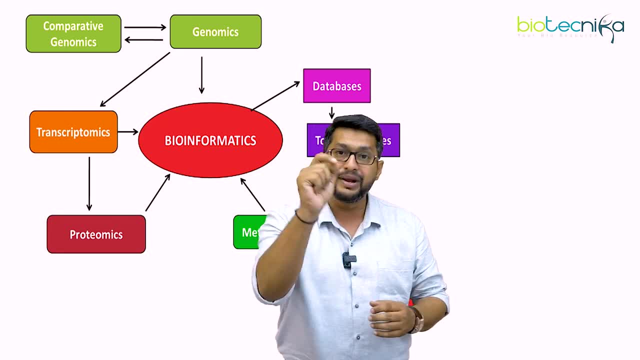 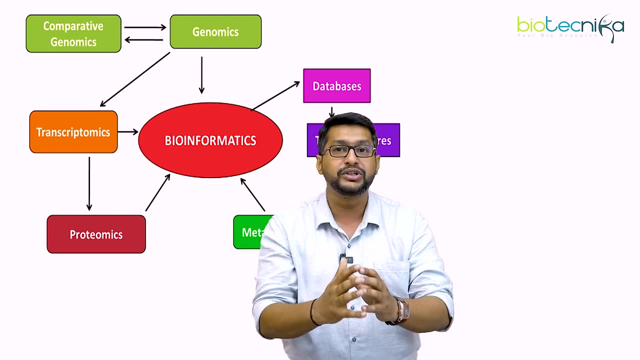 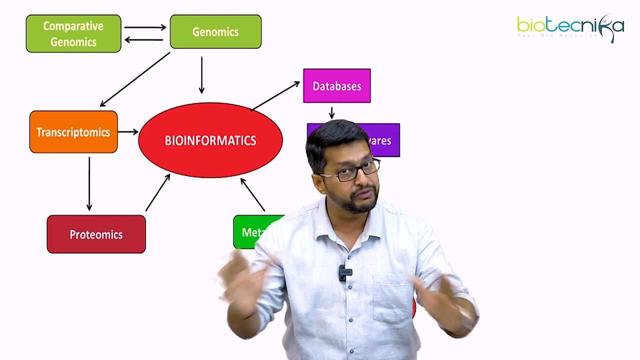 And what is the modulation pattern of a particular gene could be understood with transcriptomics. However, at the end, we know That every gene produces a particular protein, and this protein is the end product. Now, protein folding, protein stability, protein functioning and protein bioactivity plays a very, very crucial role in any organism. 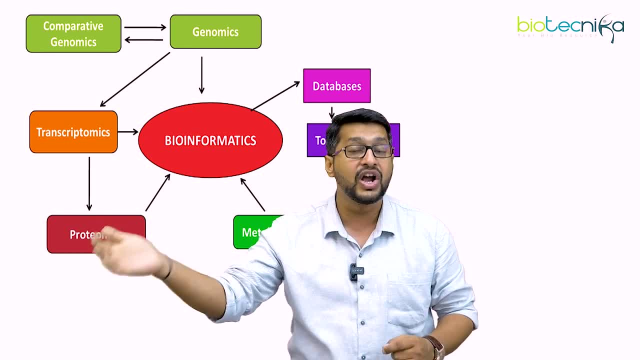 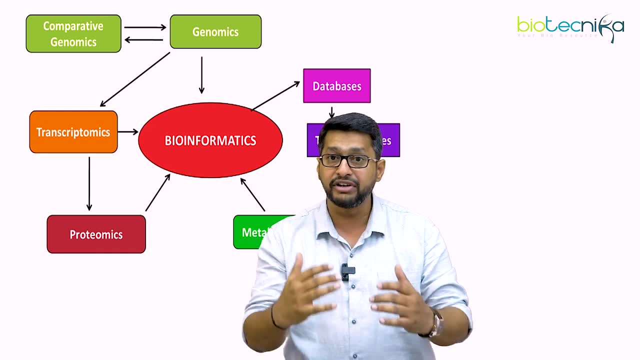 And hence understanding this in terms of biotechnology and in terms of bioinformatics becomes very, very crucial. Now, this was just a classical central dogma, But, however, in modern central dogma, we all know that you know proceeding forward with that of the protein. 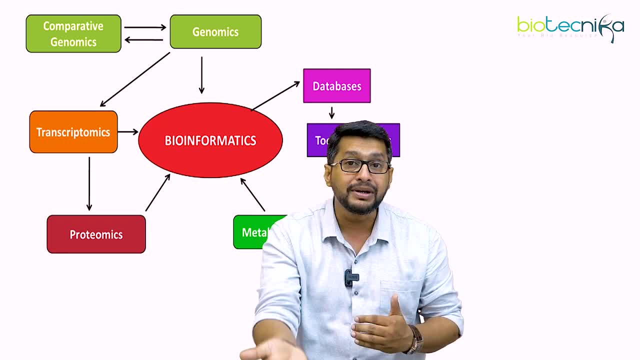 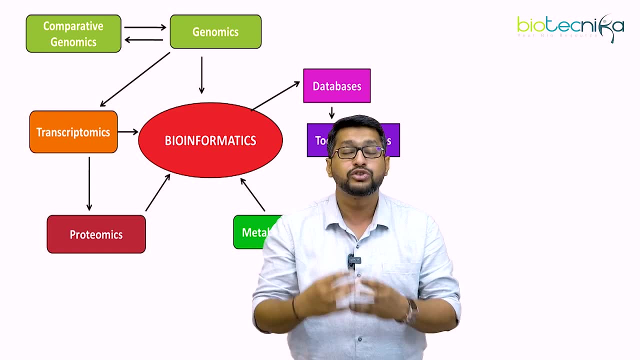 You have something which is called Metabolome, that is, you have a metabolite which is coming from this particular protein. Either it could be a primary metabolite, secondary metabolite and tertiary metabolite, And these metabolites could be used for human welfare. 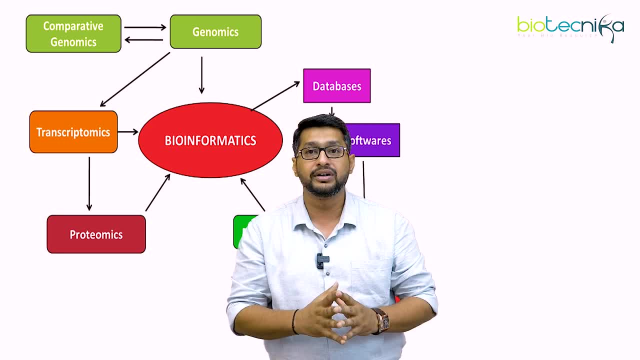 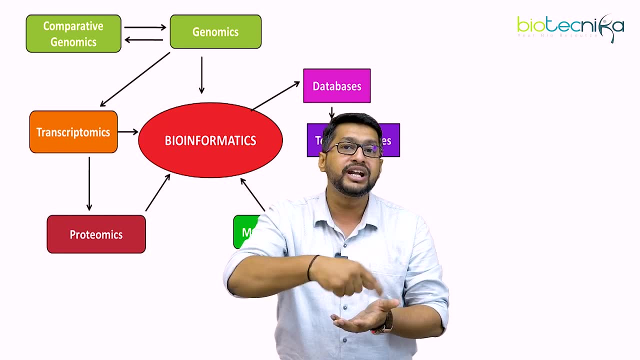 So, hence, understanding the metabolomic part of it is very, very crucial. Now, please remember, bioinformatics is just like a toolkit, So I can use this particular toolkit for understanding various kinds of biosystems. Either it could be a plant, it could be a microbe, it could be human, it could be an animal. 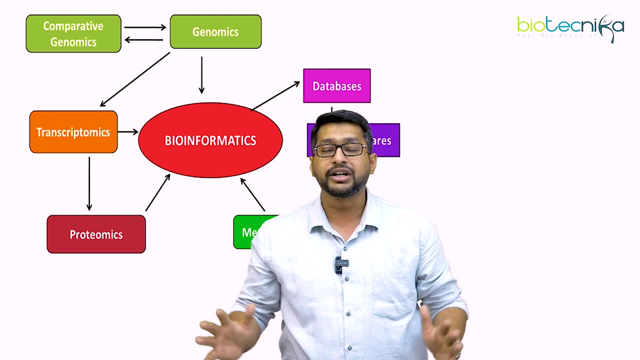 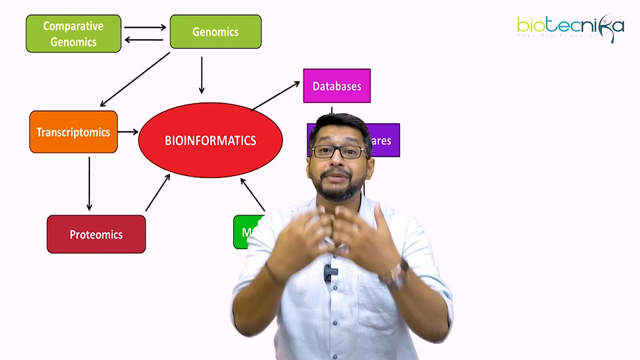 It could be a road, It could be an aquatic organism, whatever. But however you know, the tool remains the same, but only the differences with the bioorganism which we are trying to implicate, the rules of this particular tool, or the package or the software to understand those organisms in a much better way. 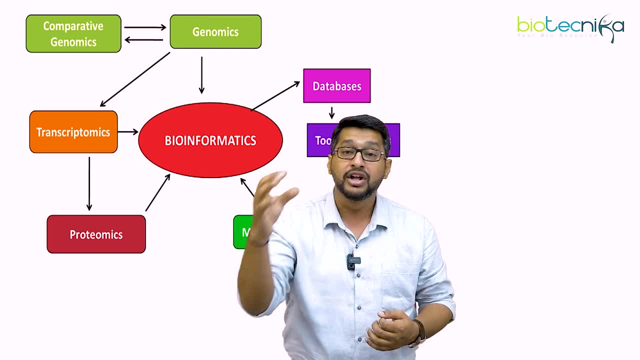 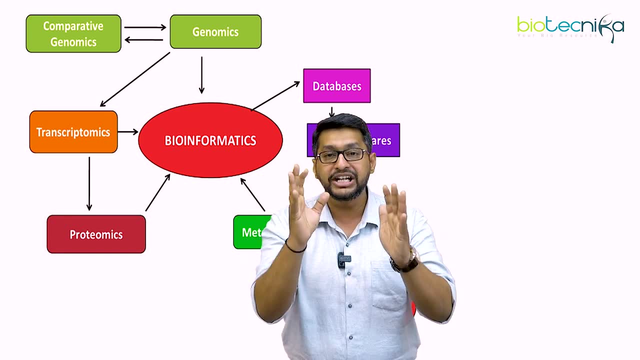 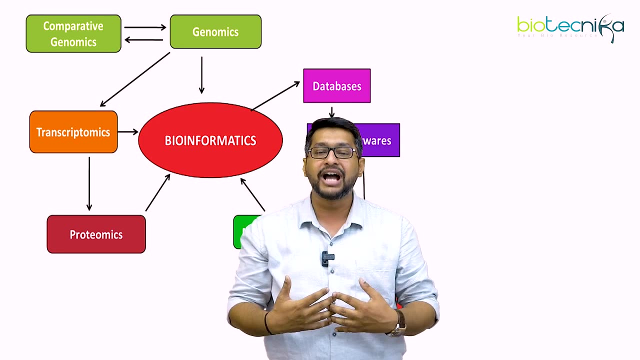 So, with these particular tools, softwares and packages, what you get is you get the desired results. Now, these desired results. remember, these are predictions. now, in 80 to 85 percent of the cases, these predictions are actually right. However, you need to always validate it before you try to have a bigger claim. 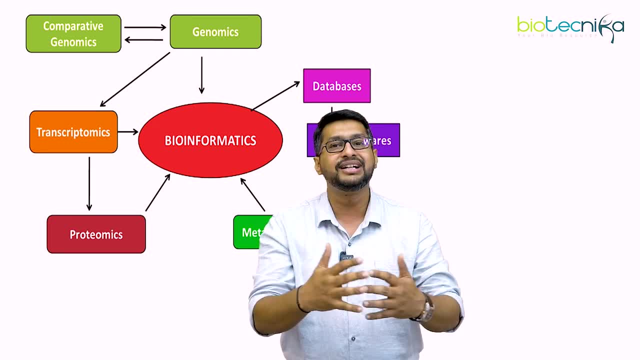 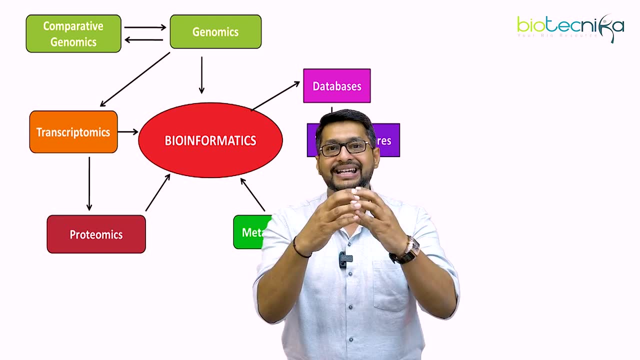 You need to always validate bioinformatics, OK, and once you validate it using your wet lab experiment, that is where you know your bioinformatics and your biotechnology has a concrete idea And this is how it emerges into a newer and interesting results. 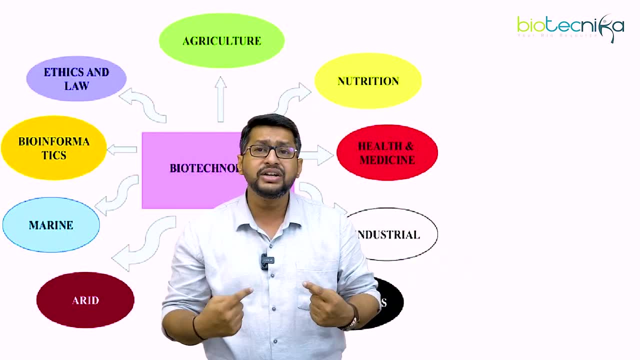 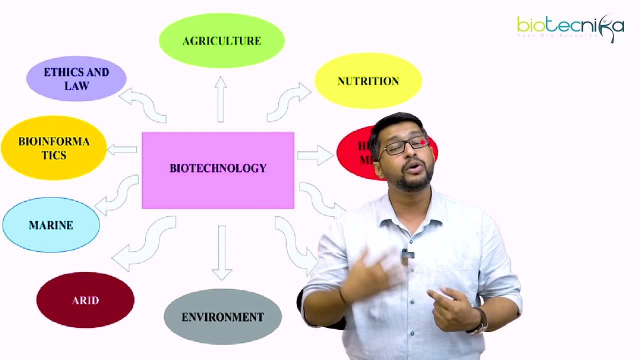 Now, with these new combinations, what are the various branch of science, or branch of biology, which could be actually explored? now, a greater component, Because most of our students- OK, they talk about. Sir, I want to use the applications of biotechnology in agriculture. 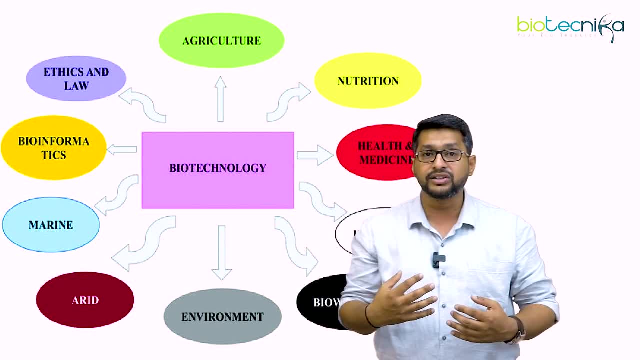 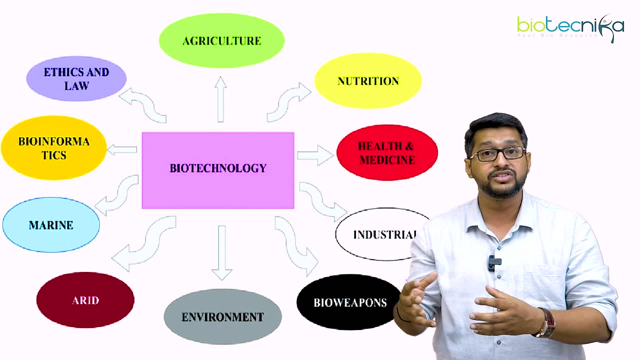 So here is what a new branch which is called as agriculture biotechnology- You can talk about nutritional biotechnology. You can talk about health and medicine. You can talk about industrial biotechnology. The other one is bioweapon. I do not, you know, try to give a lot of illustrations on it. 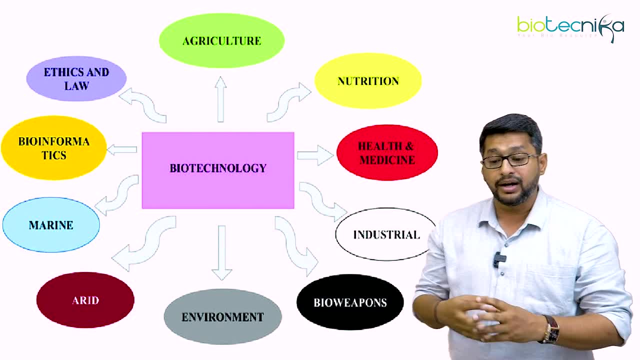 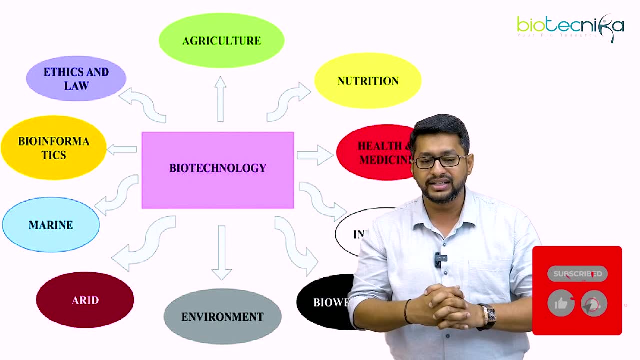 But yes, bioweapon is also one of the major component. You have the environmental biotechnology, You have the arid biotechnology, You have marine biotechnology, huge scope in terms of- you know the current scenario- marine biotechnology. 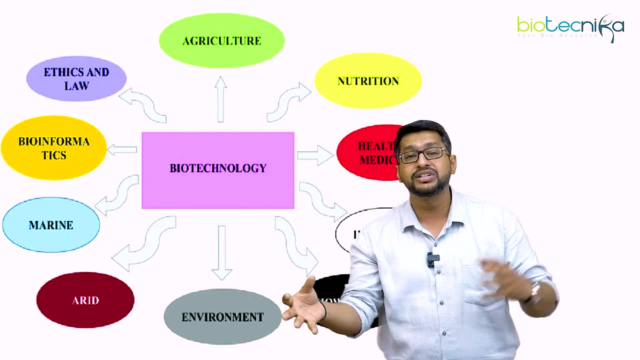 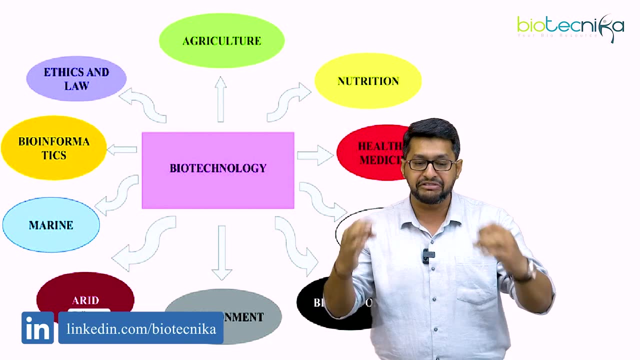 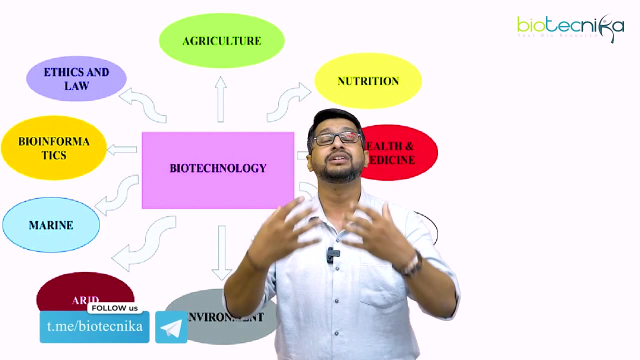 Then you have the applications of biotechnology in bioinformatics and bioinformatics into biotechnology, so that newer and newer science have been developed every day, every minute, every second, And very, very important. I should also understand: once I have a discovery or an invention, how do I make it under my particular name? 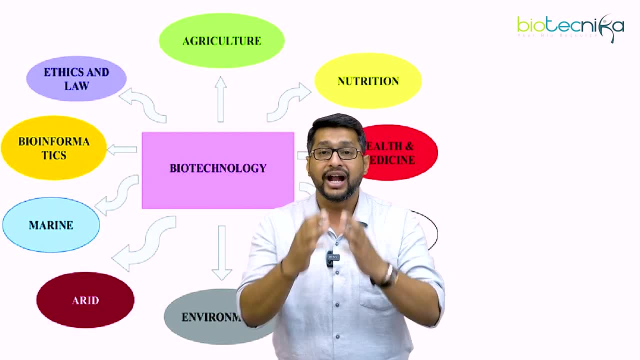 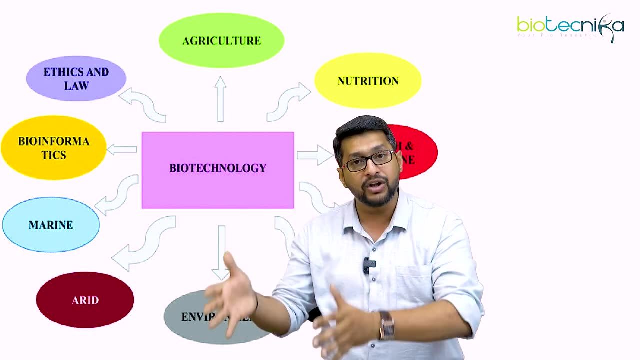 So I need to also understand the proprietary of my research And to understand this. This is proprietary. The law and ethics plays a very, very important role And hence ethics. when it is applied onto biotechnology, it is called as bioethics and law which has been applied onto biotechnology. 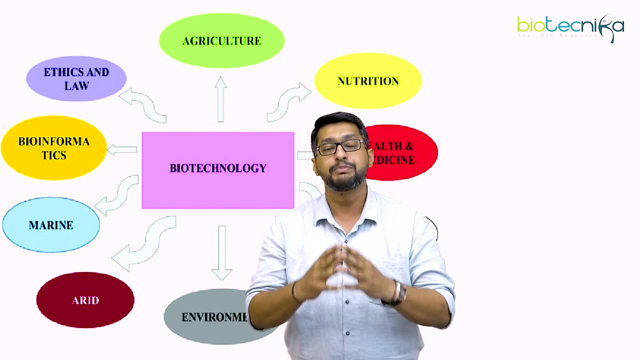 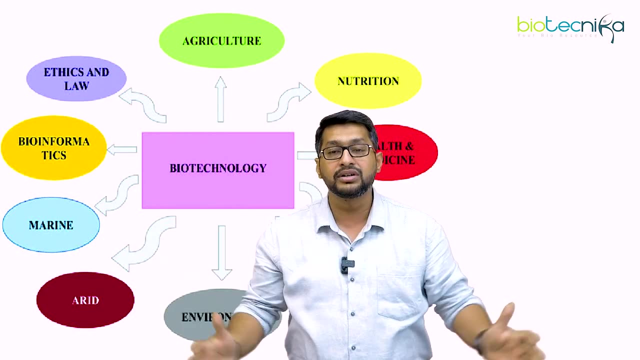 It is called as IPR. The IPR refers to intellectual property rights, So all these branches plays a very, very important role. Please remember, my dear friends, all these disciplines are booming up. It has a lot of scope. So just think out of the box. 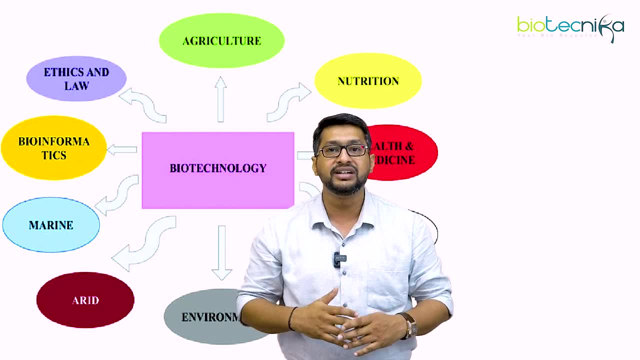 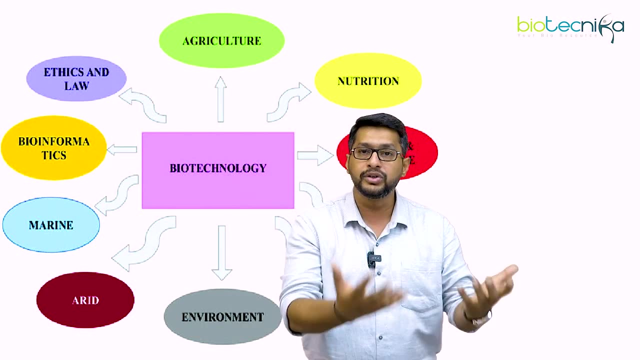 And when you think out of the box, This is where innovation and creativity has been kindled, And that is where you come out with a new product which could be either patentable, or it can go for a manuscript or a publication or, you know, you can go for a copyright. 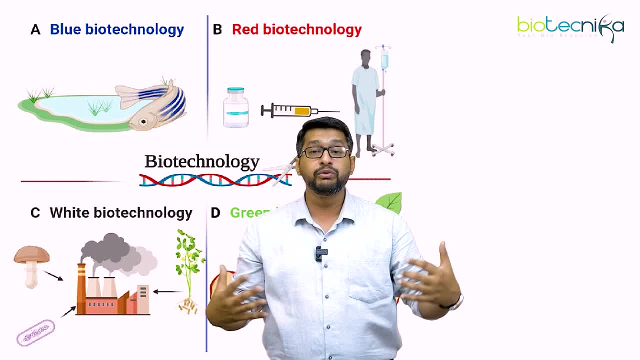 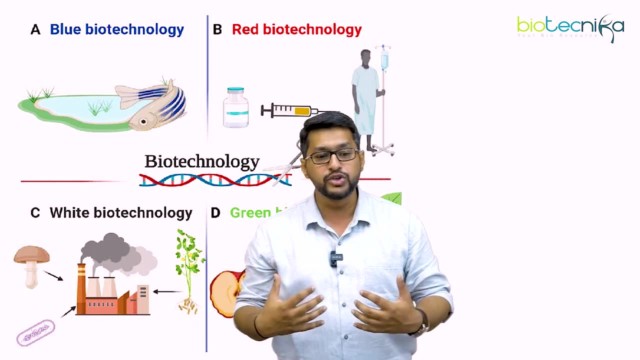 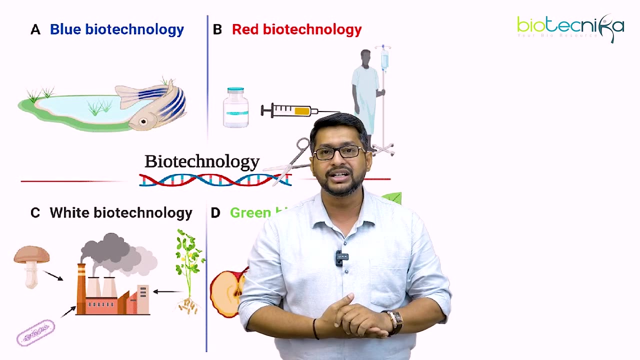 Now, what is the evolution of biotechnology? Now, when you look into the evolution of biotechnology, there are four major evolutions, what I have seen. So the first evolution was in terms of blue technology, wherein people were like extraordinary, focused with, you know, the water and the marine technologies. 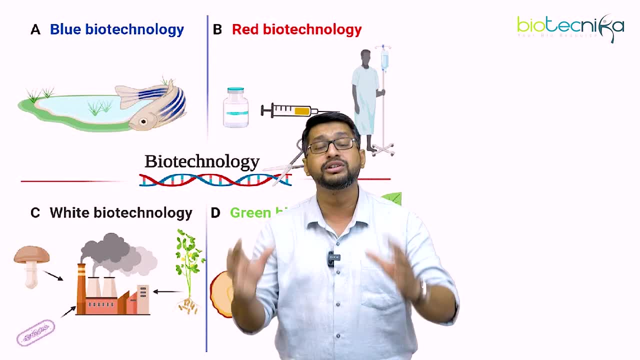 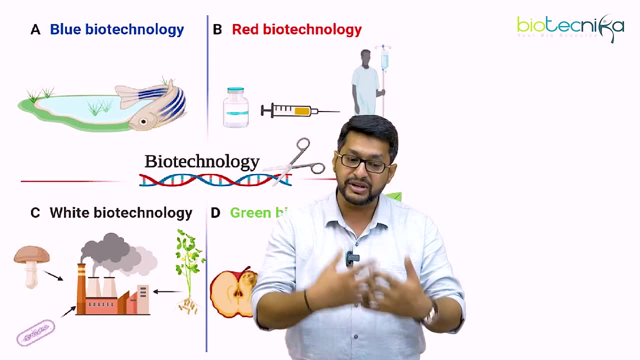 Then it came on to the earth, on to the red technology, wherein human health was the major priority in the under red biotechnology. and then you had something which is called, as you know, industrialization, especially with white biotechnology, wherein you know various kinds of metabolites, you know milk, all these kind of 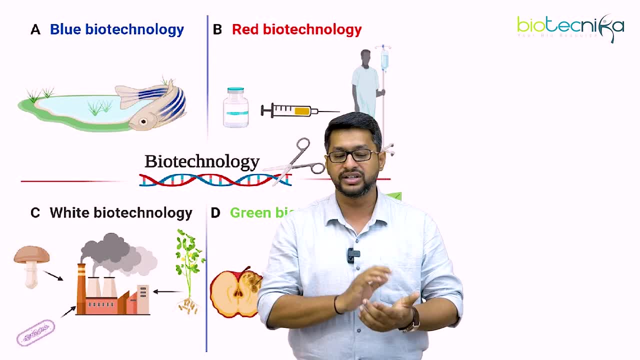 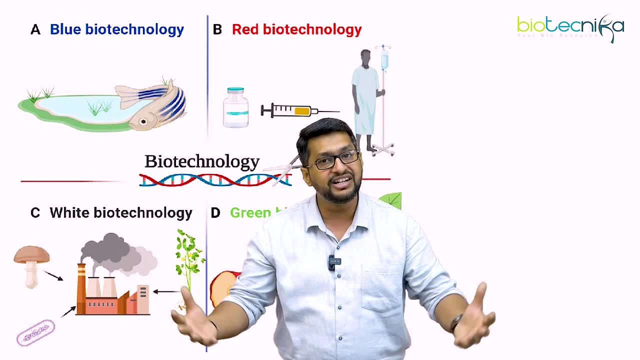 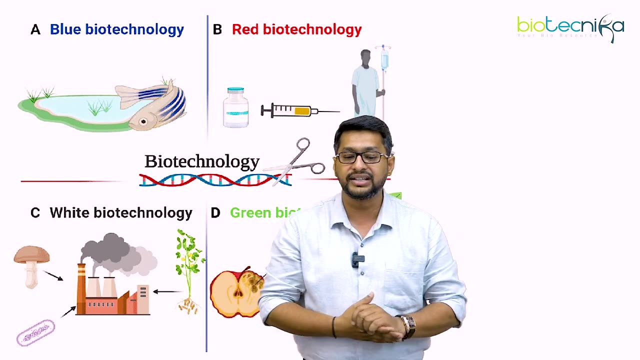 industrial products were explored. and this is where your white biotechnology comes into picture. and, not to forget, you have green biotechnology, wherein new crop variety, new breeds, new crosses, all these were developed. disease resistant variety, drought resistant variety, all these were generated during. you know your green, green biotechnology. but, however, now we stand at a point. 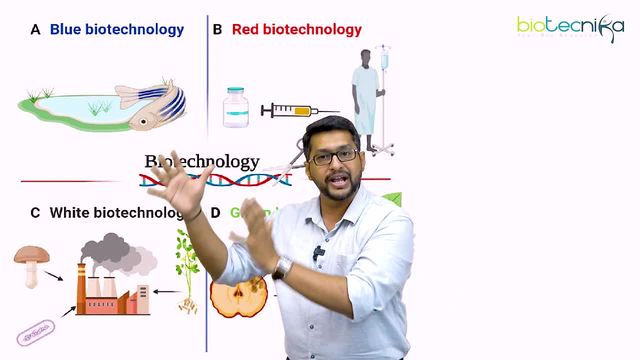 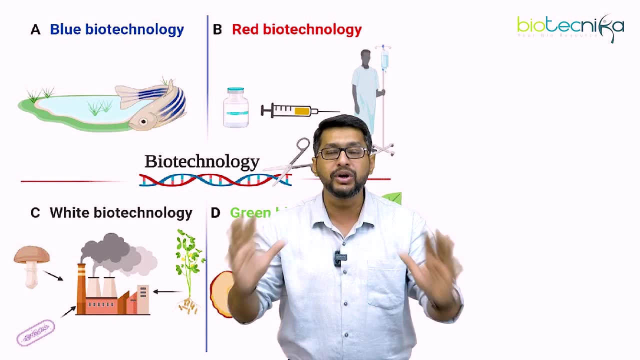 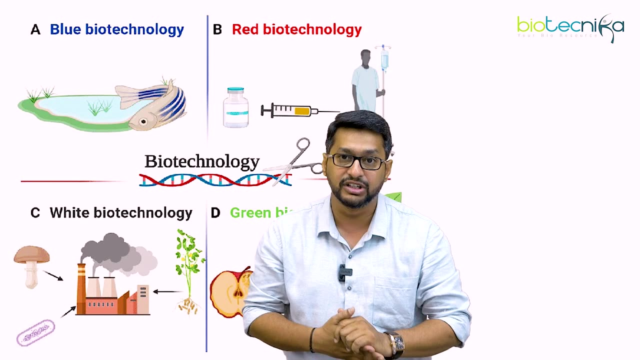 wherein this entire biotechnology is meeting bioinformatics. now, when bioinformatics meets biotechnology, there is a boom, and this boom has led into a newer biotechnology, and this newer biotechnology has led into a great revolution, and this revolution is called as the data revolution. so now, 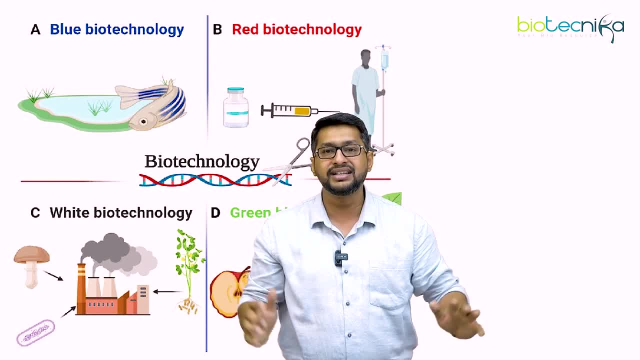 we are standing at a point wherein data is everything. either it could be your personal data in terms of your fingerprint or your iris scan, but however it could be, here the major emphasis is on your bio data. okay, so once you have the biological data which has been screened, 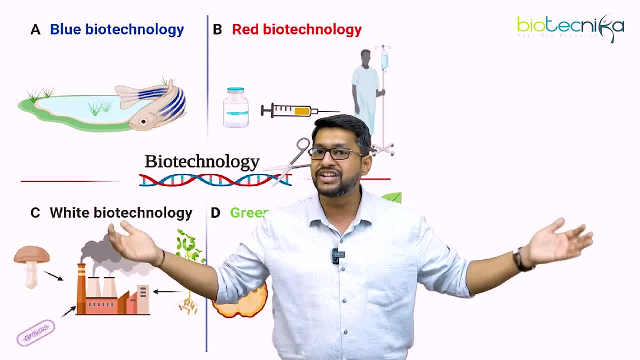 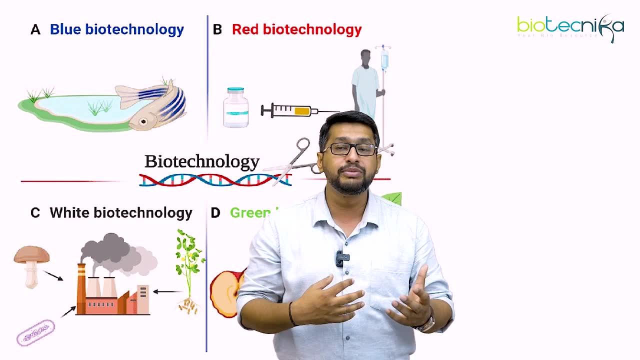 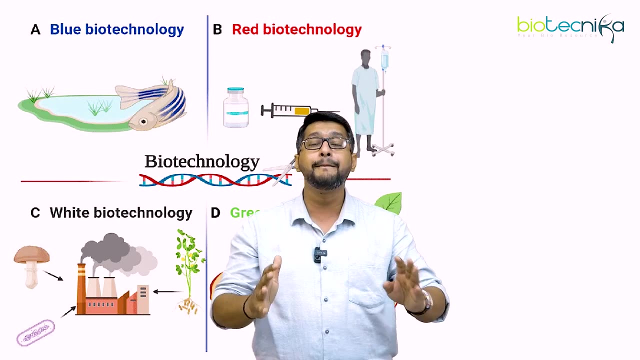 either your proteome has been screened or your entire genome has been screened. now this acts as your data. okay, so this data could be used for security systems. this data has been used for identification systems. this data could be used for various kinds of disease and diagnosis, and people are now have been crazy enough to look upon this particular genome and 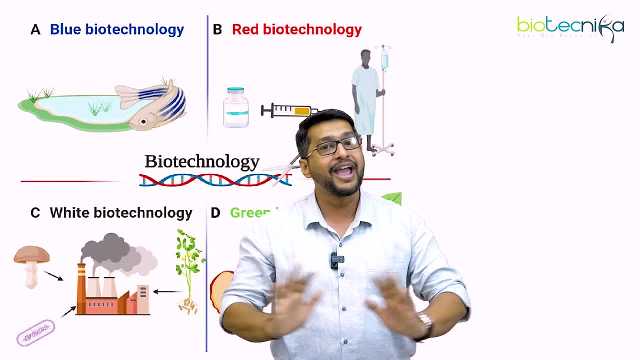 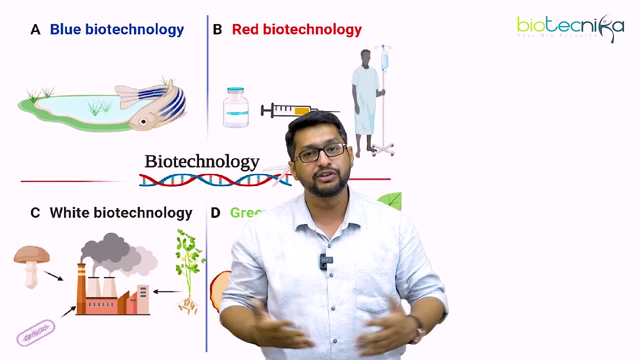 predict when exactly they die. so, trust me, my dear friends, now everybody has money, but nobody wants to die with this. okay, people want to predict their death? okay, by measuring various kinds of you know, biomarkers from telomeres etc, etc. okay, so this is how you know your genomic data could. 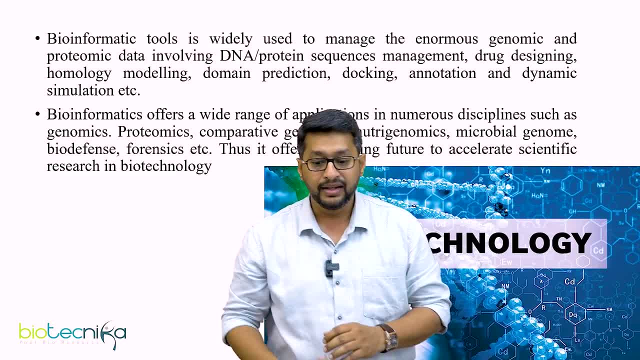 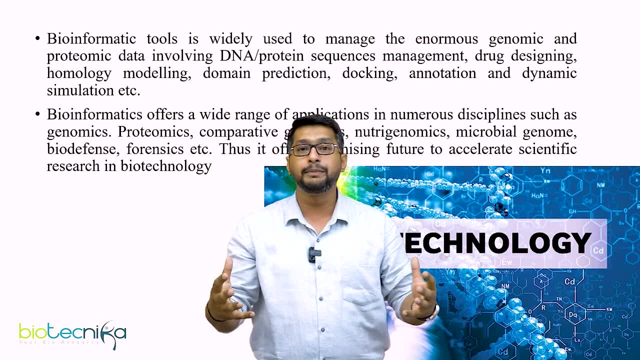 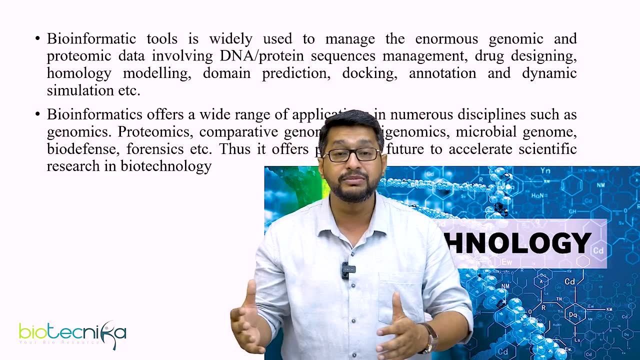 be either explored or exploited. now, with this, people has come up with new biotechnology, what we have not mentioned previously. the newer component is understanding the- you know uh, the dna protein sequencing management, understanding the drug design management, understanding the homology abinsure methods, domain productions, annotations and 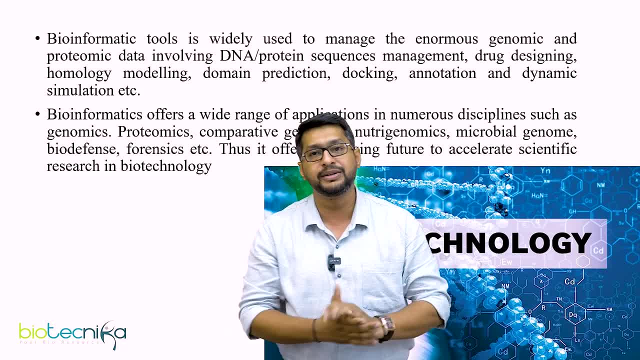 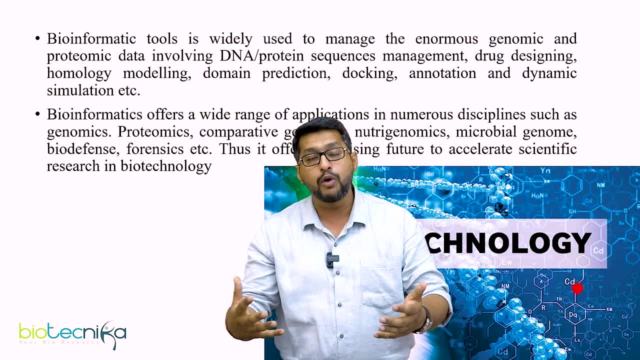 dynamic simulation studies could be very easily done using bioinformatics, so that you can have a greater impact on biotechnological understanding. now, moving on forward, you have nutrigenomics, a fantastic branch which will understand the genealogy and the genealogy of the genome, and 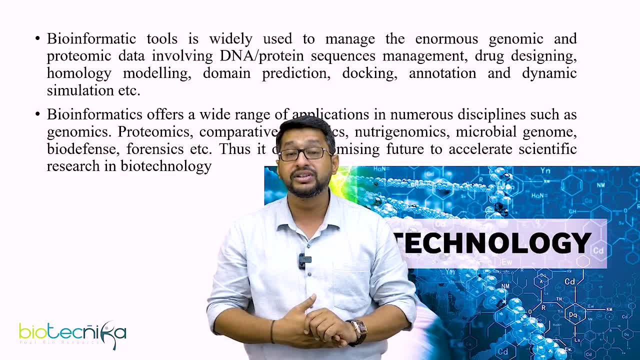 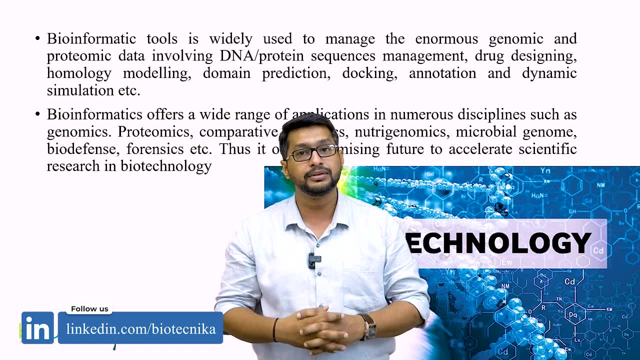 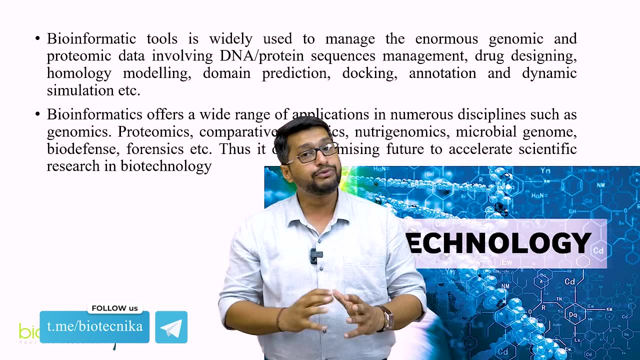 genomics and that of nutrition. so this is called a nutrigenomics microbial genome. uh, very importantly, in terms of microbiota, okay, or microbiome research, which is like the, the booming component, and, very importantly, we can use the laws of bioinformatics in forensic science. now, in forensic science, you, 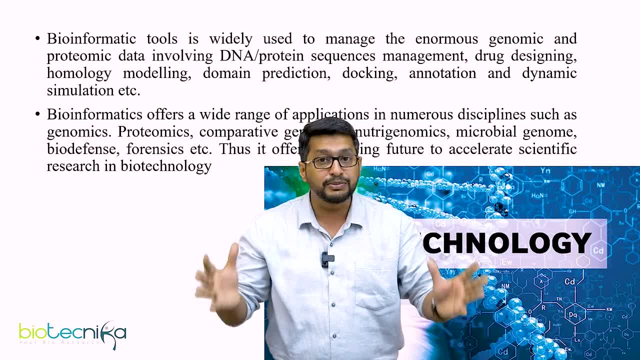 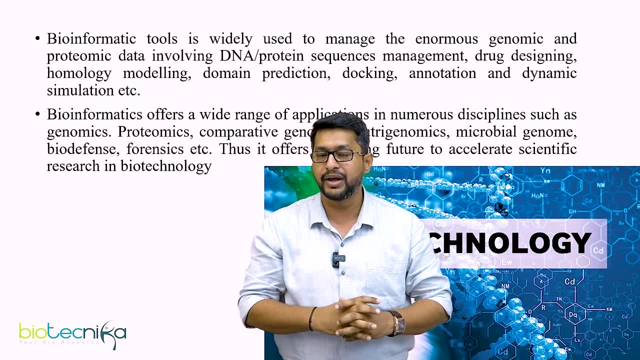 know, depending on what exactly is your case. okay, you can actually explore the power of bioinformatics in biotechnology. so, uh, the the ultimate line. what if you? you know, if i am suggesting something to you, the ultimate line or the ultimate conclusion? what i am trying to make you understand is: this is a 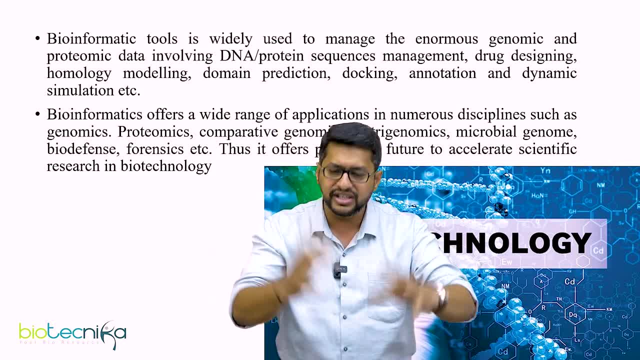 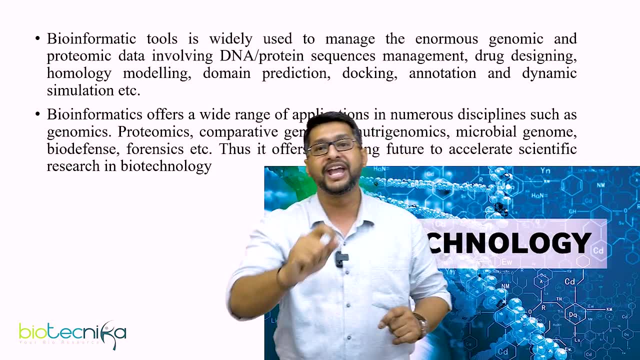 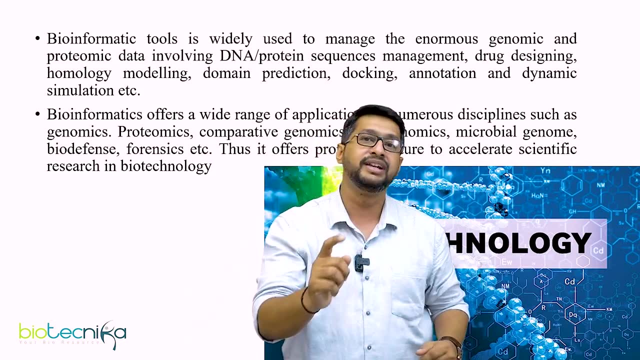 very, very promising technology. this offers a promising future to accelerate the scientific research, especially in biotechnology. so i urge, i appeal all my young friends to take up research as one of the major component, because the next 10 years, especially in india, research will dominate. okay, a government is trying to put up a lot of funds, uh at, uh you know, degree level at master. 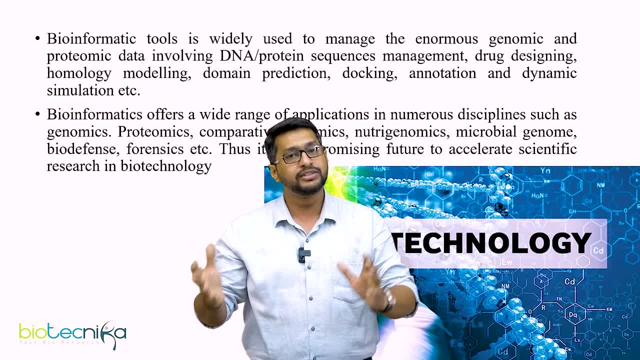 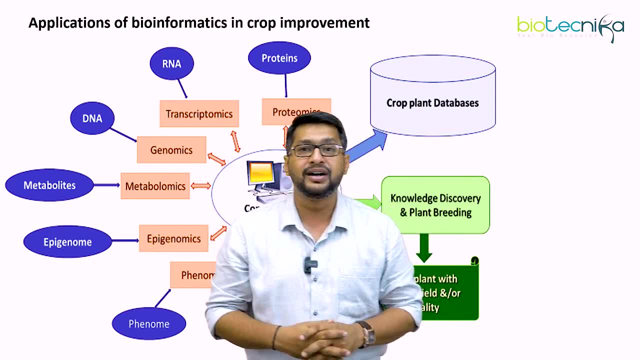 degree level and at a uh degree level, at a master degree level, at a master degree level and at a phd and a postdoctoral level. so please utilize this facility now. uh, most of my students, when they actually, you know, try to come into the internship. okay, or they are doing certain. 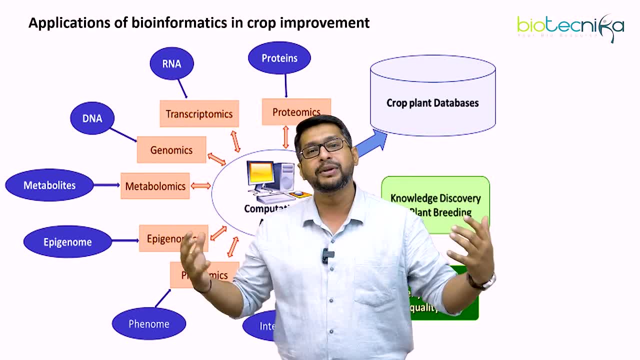 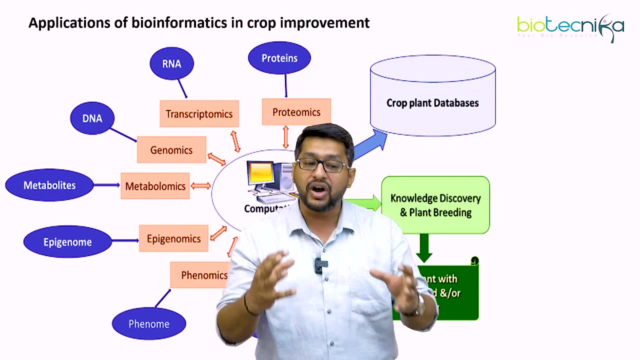 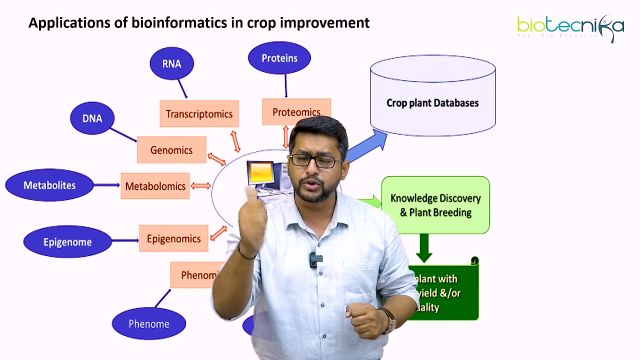 certification courses at biotechnica. they ask a very common question: sir, how do i use the laws of bioinformatics, especially in agriculture? so here is an important illustration which talks about the application of bioinformatics in crop improvement. so here either, i can look into the, the protein. 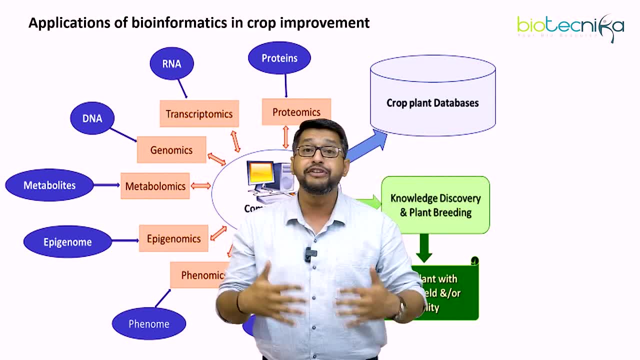 DNA component, metabolomic component, epigenomic component, a phenomic component or interactome component. okay, and when i look into this, i can- i can still use the laws of bioinformatics and this is called as computational analysis, and this computational analysis will help me in creating. 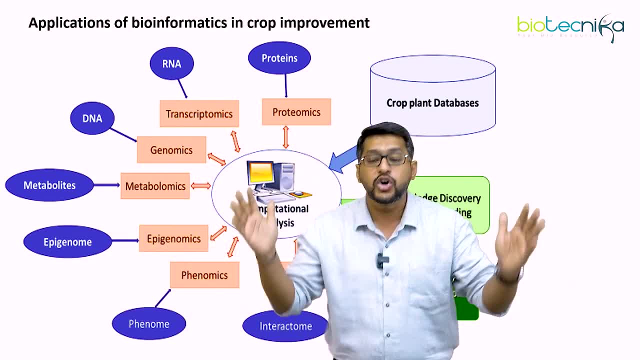 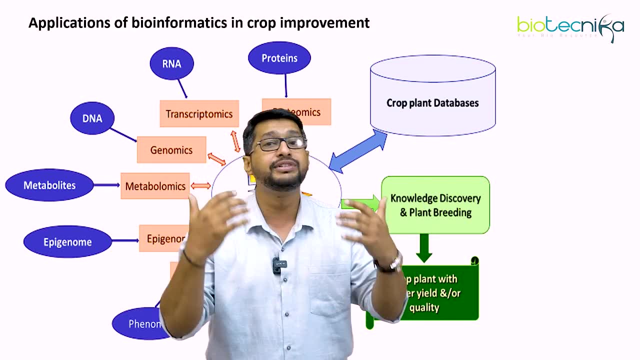 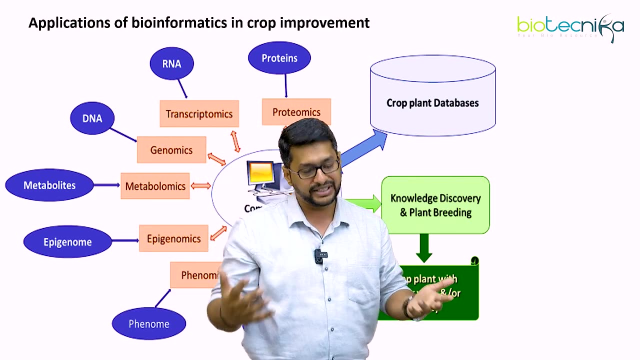 a huge database and this huge database is called as crop plant database. when i talk about crop plant database, this will actually enhance the knowledge discovery of the plant breeding and then, very quickly, i can lead into, you know, crop plant with a better yield and a better quality. now, if you 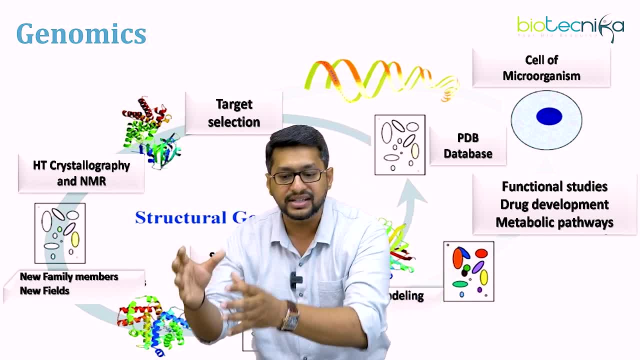 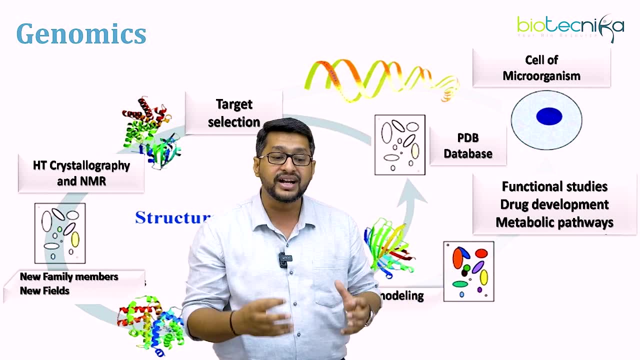 look into the, the genomics you know. just to give you an illustration, imagine that i have a particular cell and from this particular cell i am trying to isolate a selected target. and once i have the selected target, i can go for various kinds of crystallographic analysis for the selection of. 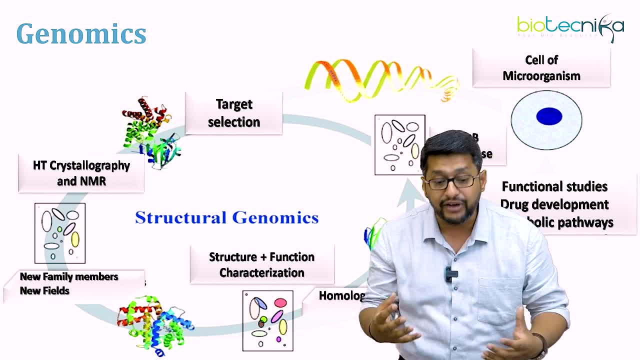 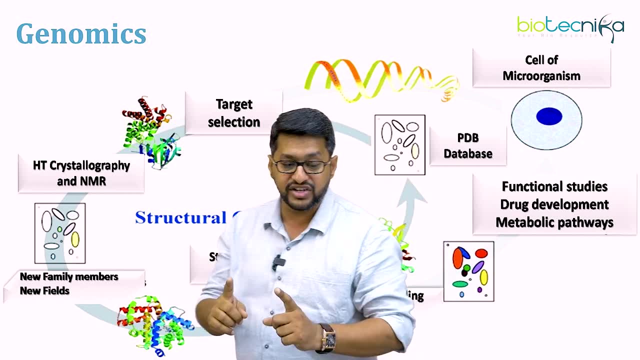 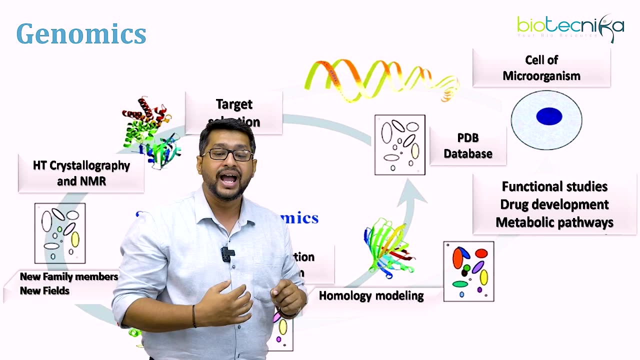 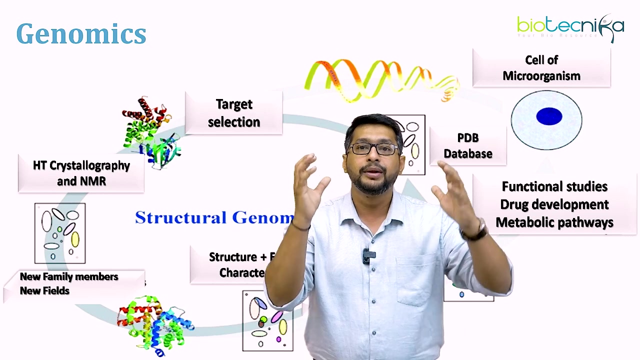 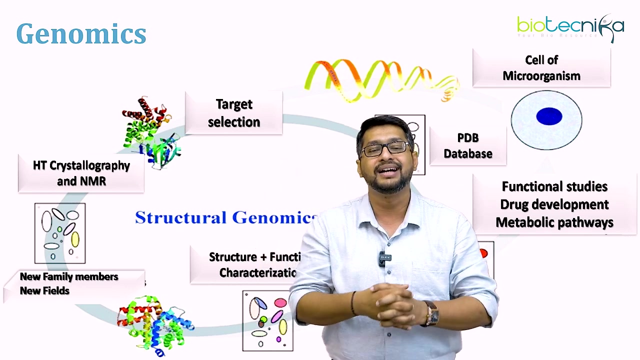 that bio target and then i can look upon this target belongs to what family of the proteins? and with this protein family i can look for function and functional characterization. after that i can go for structural and functional characterization, and when i look into the structure and the functional characterization, later i can go into homology modeling and with homology modeling i can go for functional studies, drug development and metabolic pathway development. this creates a huge impact on the farmers, on the agricultural scientists, and this can be created into a base and this is called as a crop, or you know. you can. you can call it as a microbe database or you can called as plant database, or you can call it as plant database or you can call it as micro pursuing disease. but even the overseas- i am only talking about it because i'm going to describe it. uh, now there's some species, elderly disease, so it's not working. 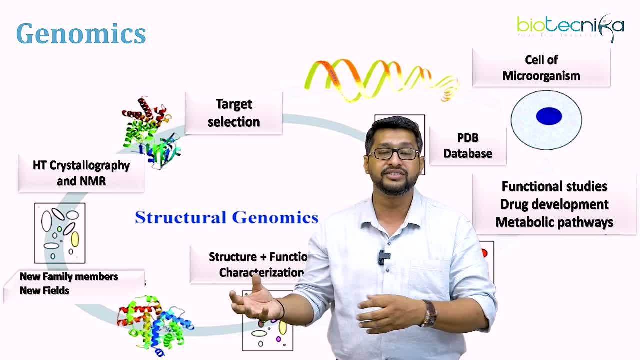 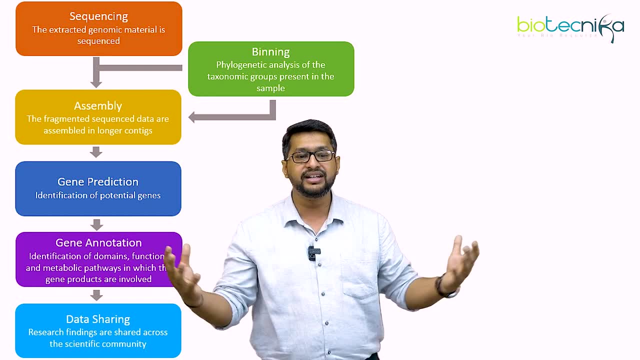 you can call it as a protein database specially dedicated towards plants, so you can have various kinds of combination of databases. now, how is this been done? this has been done very, very easily. that is, you know, you start extracting genome, genome and then you sequence it. once you do. 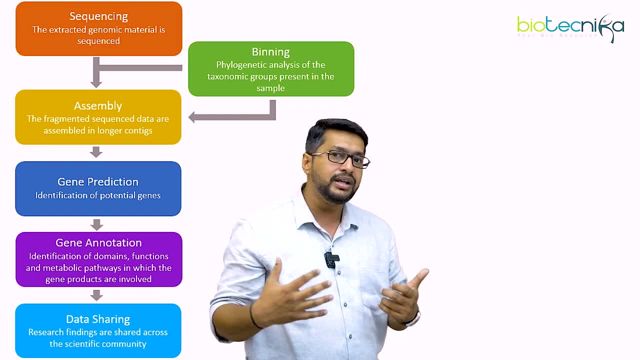 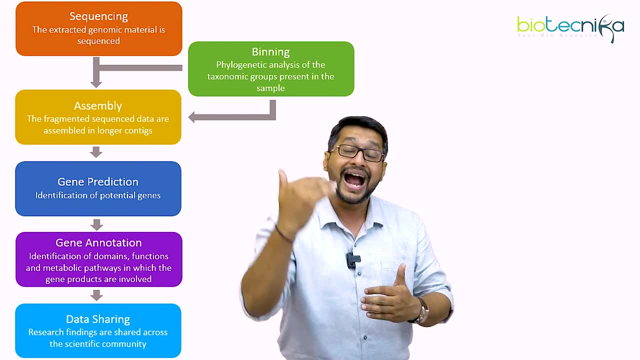 that you can create an assembly, and before you create an assembly you can actually look into the binning component, wherein you can create the phylogenetic relationship with the sequences- what you have got and the sequences which are already available in the database- and then you can go for. 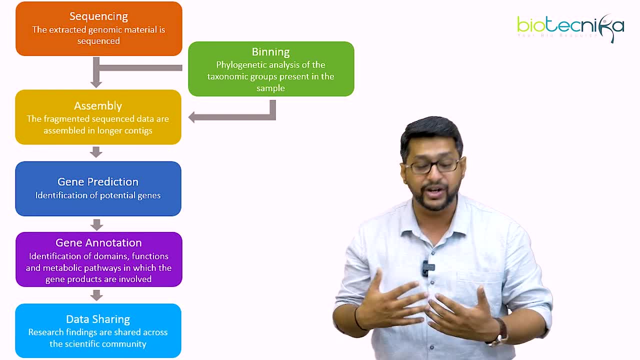 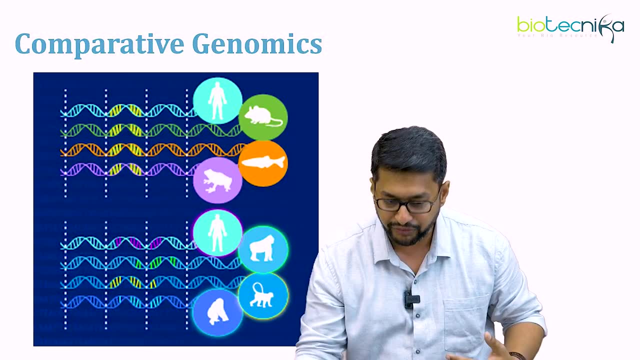 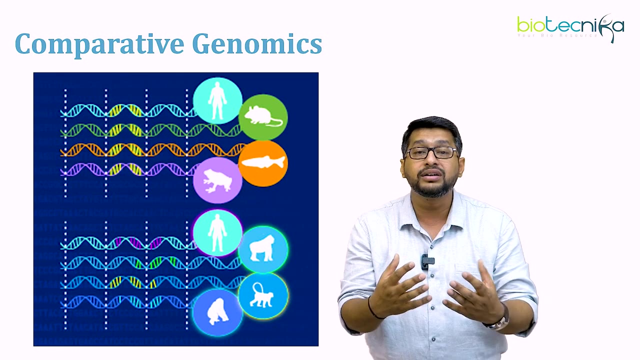 gene production and with the gene production you can also look for gene annotation. and once you have the gene annotation, the data is already there for the entire scientific fraternity to utilize it for the welfare of humans. now i was talking about, you know, comparative genomics. now, once i have the data, now it becomes very, very important that i am not interested in looking into. 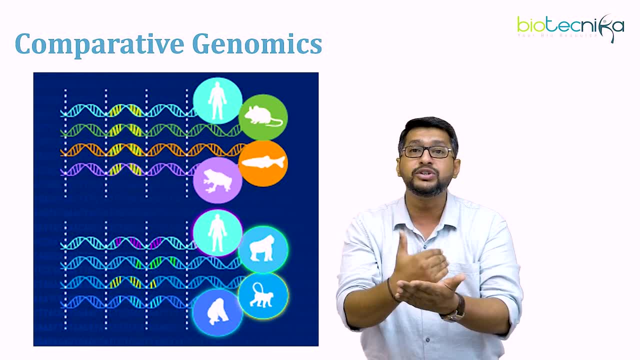 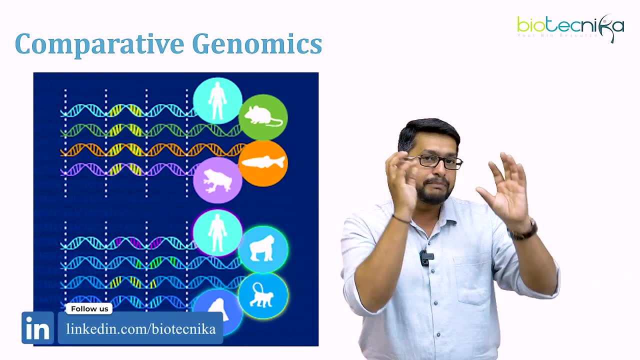 an individual or species specific data. i want to look into a data which has like cross species data. so when i look into the cross species data, i want to look into what are these microorganisms doing in humans? what is the same microorganism doing in a rodent or a mouse model, or 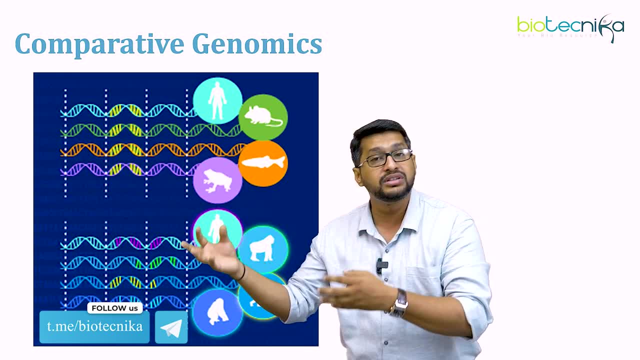 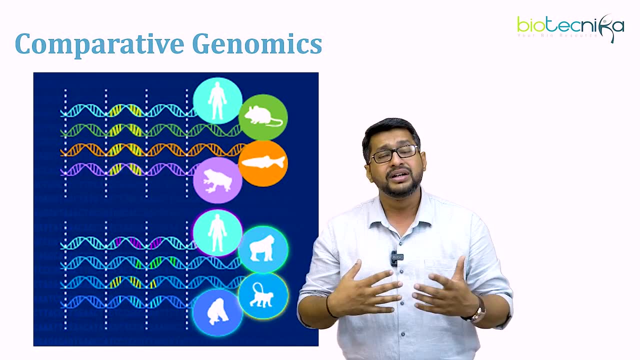 a murine model, then what is the same microorganism doing with, you know, the fish model? or i can go for what are the various kinds of amphibians, or various kinds of plant? you know, you know, it is all. depending on the level of creativity and the way you think out of the box, that can lead into a 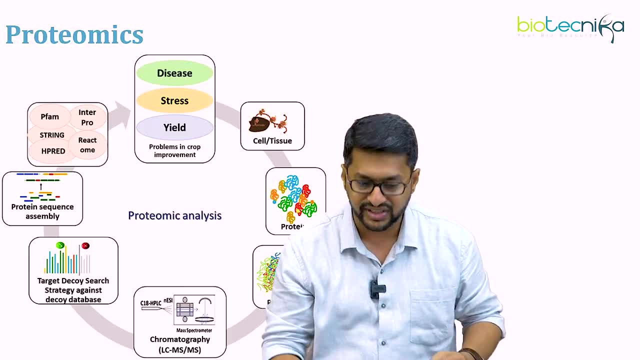 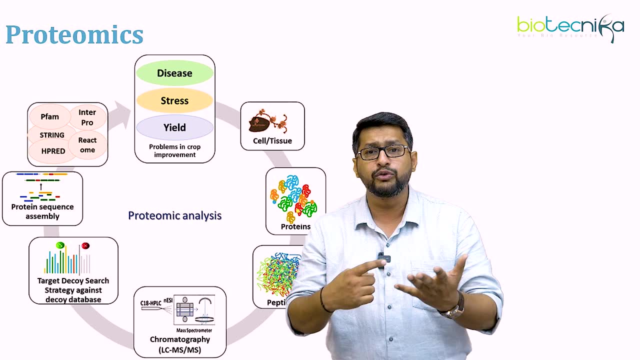 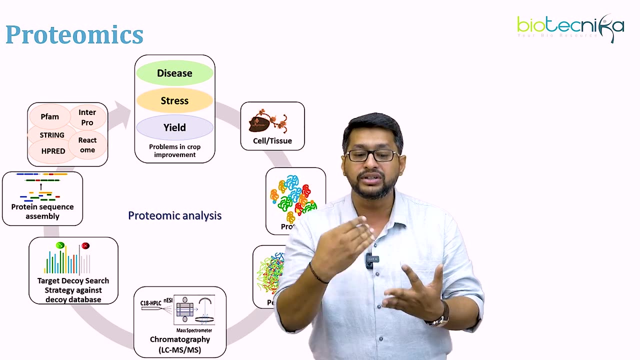 various kinds of results and especially comparative genomics is one such approach. now, finally, you can approach wherein, especially, you can look for various kinds of diseases, you can look for various kinds of stress factors, you can look for various problems which have been encountered. uh, for the crop, improvement in very, very much important in terms of yield, because now you know, 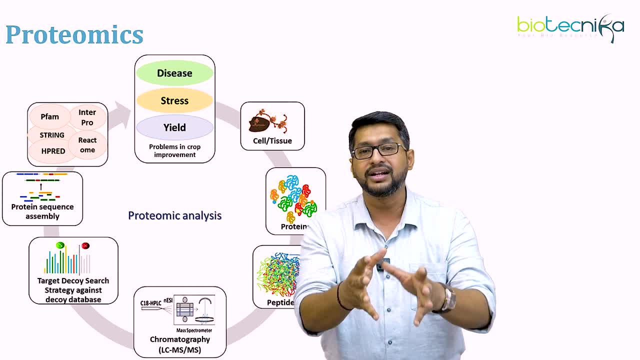 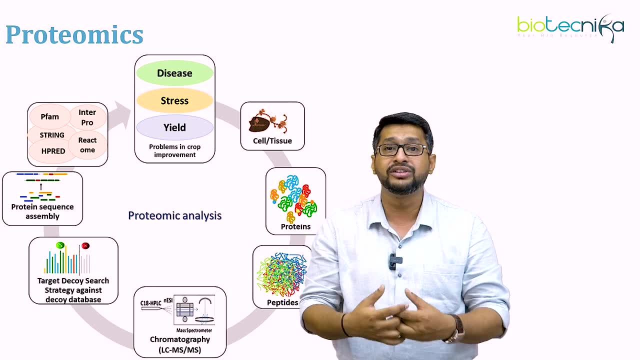 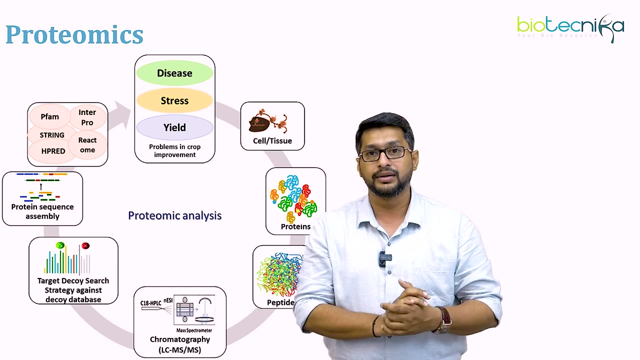 there is a population explosion and now we are into a situation wherein the the soil fertility is lost and, on the other way, the crop yield is also getting reduced. now, without adding any kinds of pesticides or insects, insecticides, how do actually improve the? improve the crop, uh crop of a given, uh, you know- season, so that this can? 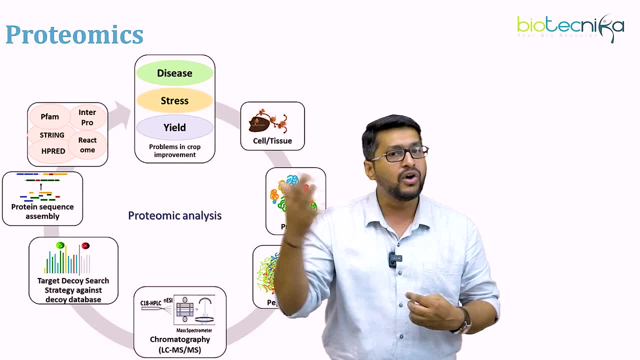 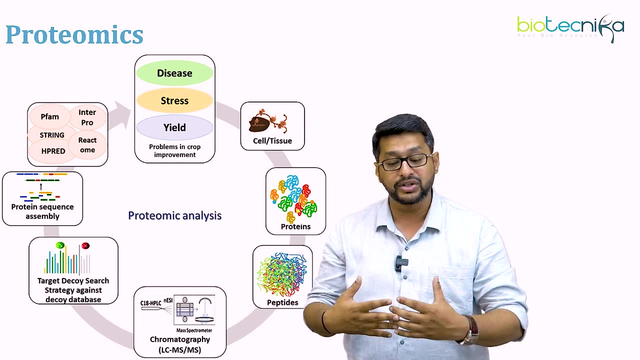 actually lead into a huge advantage to the farmer also, or or to the end consumer. so this is where you can have either tissue culture approach and from there you can isolate certain important proteins from there. from the protein you can also understand the peptides this peptides can undergo. 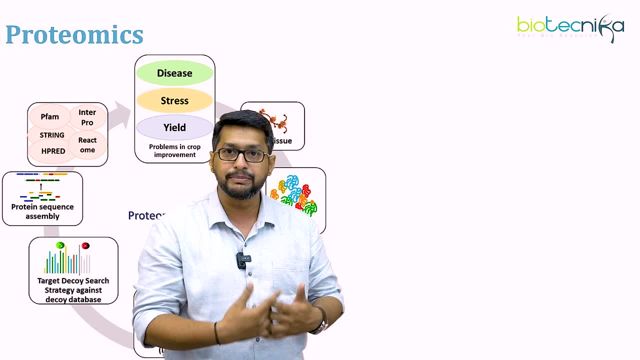 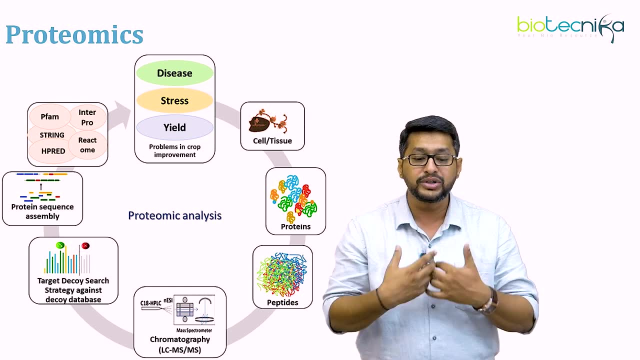 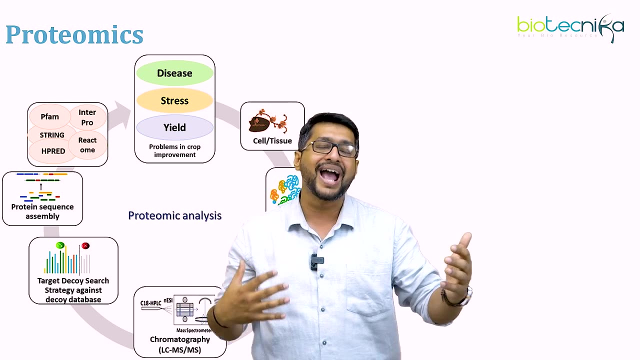 various kinds of analytical tools wherein you know you can do lcms, lcmsms, and then finally you go for the, the target identification and search, and then finally you go for a protein sequence assembly and with various kinds of databases. okay, you are able to understand. okay, how do i combat? how do i actually, you know, 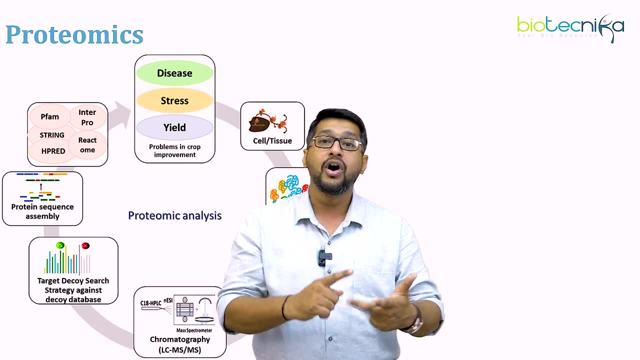 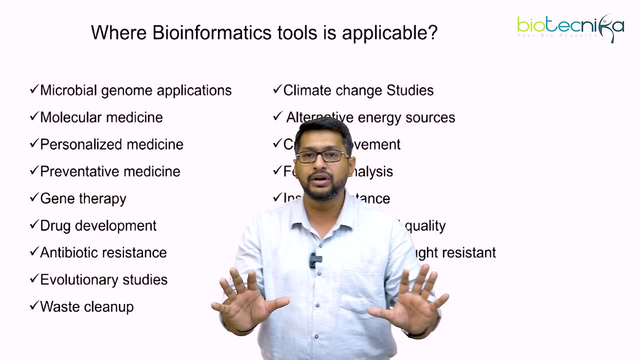 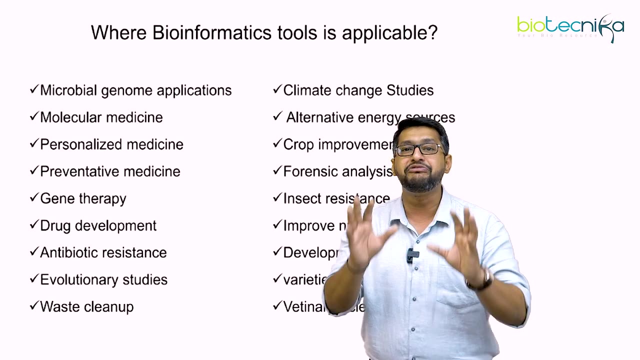 give up a solution for a disease or for stress? or how do i improve a crop of a? how do i improve a yield of a given crop? now you know, these are the. again. you know, on a very short mode, i have given you certain titles to certain captions- that these are the various 18 different fields in which 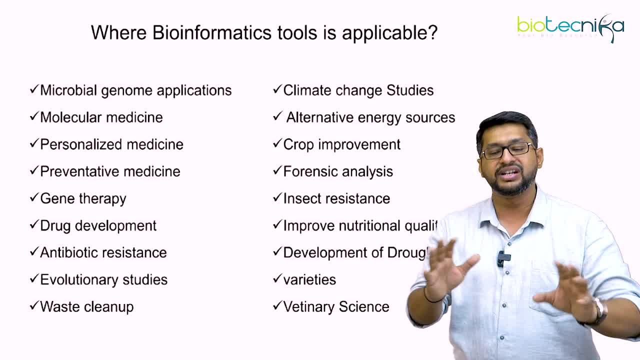 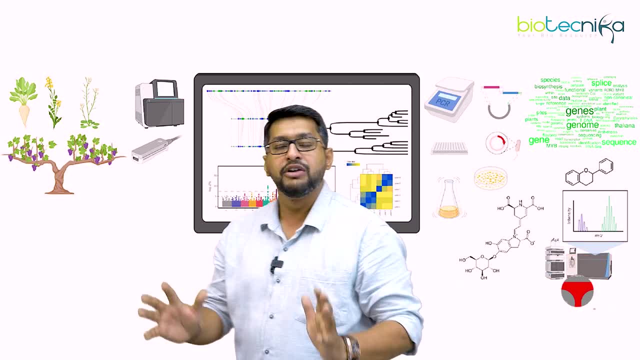 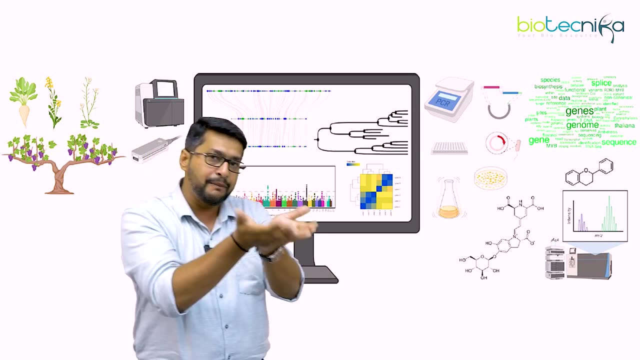 you know, bioinformatics can play an extraordinary role, especially in terms of crop improvement and crop biology. so you know, just to conclude, uh, we have biotechnology, we have understood biology and now, with this, as you know, biology and the combination of technology, you have biotechnology now and now. the only emergencies you need to use computers, and when. 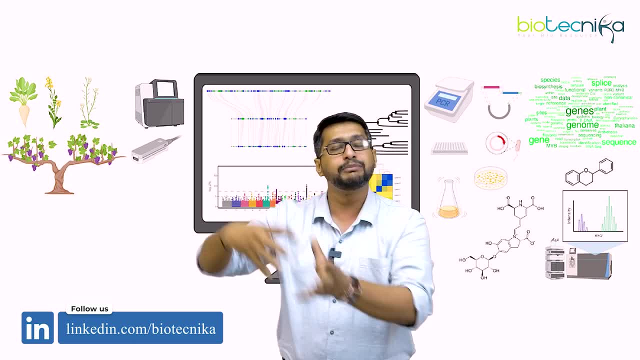 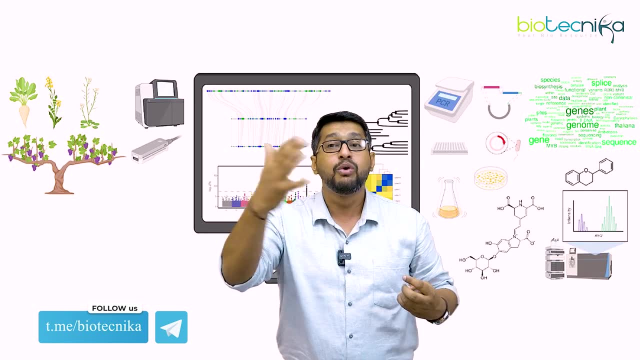 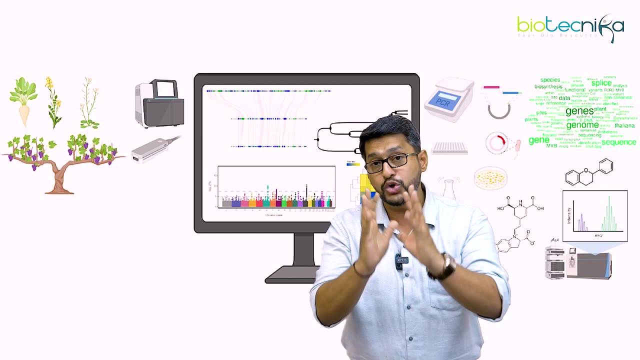 you use computers to understand this biotechnology, here comes a beautiful branch and this is like a potion. so you know you need to have a a view of what exactly you are looking at now. you know it is like identifying or searching for a needle in a haystack. so hence you, as a researcher, you should. 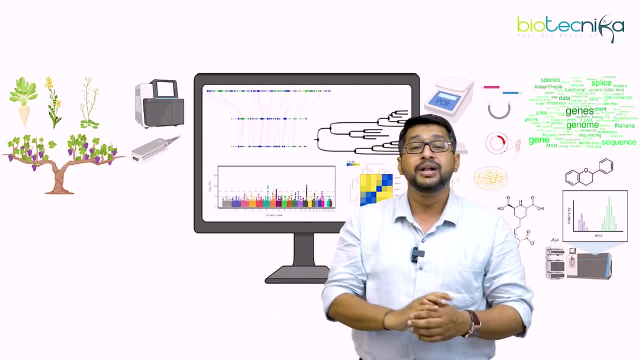 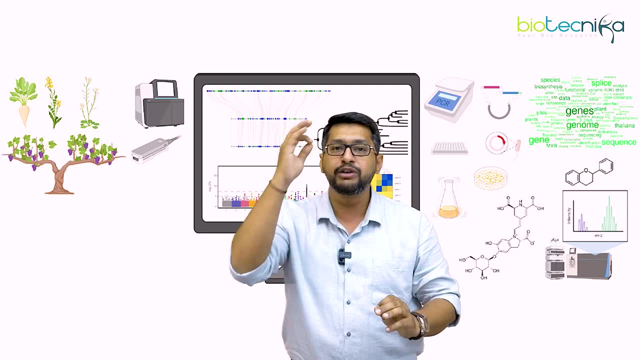 know what exactly is your focus now, without deviating from your focus. uh, trust me, my dear friends in bioinformatics and in biology, if you have patience and if you have creativity and if you are dedicated and with your perseverance, whatever you are trying to look at, look upon, 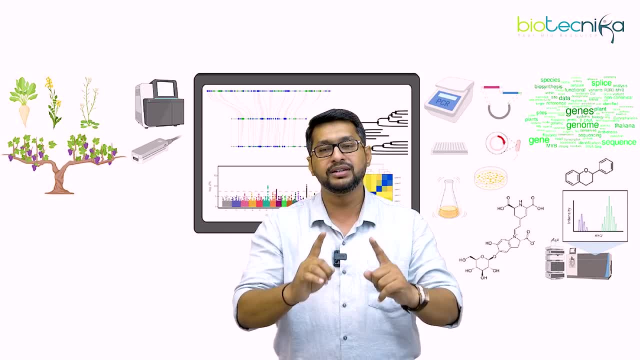 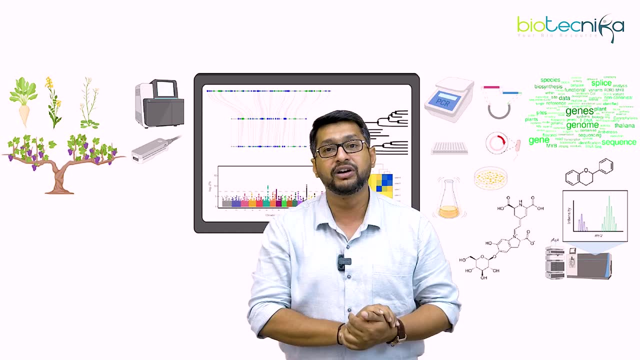 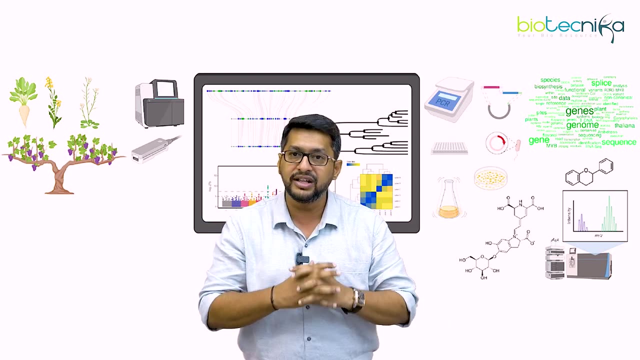 okay, you will get it. you will get it, but only time is. you know there's a time factor and also the amount of hard work which goes into that particular search makes up a difference, and your level of understanding of the concept makes a clear differentiation upon. you know, what do you actually look at? so with this, i would always 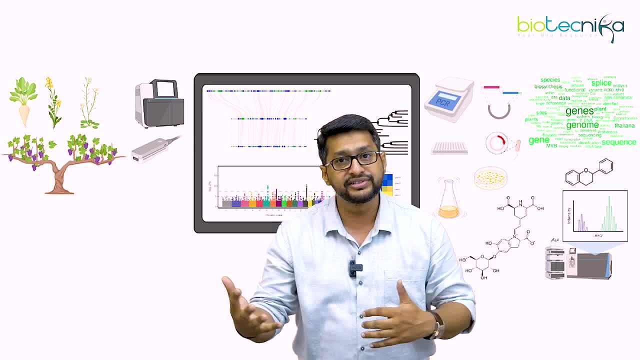 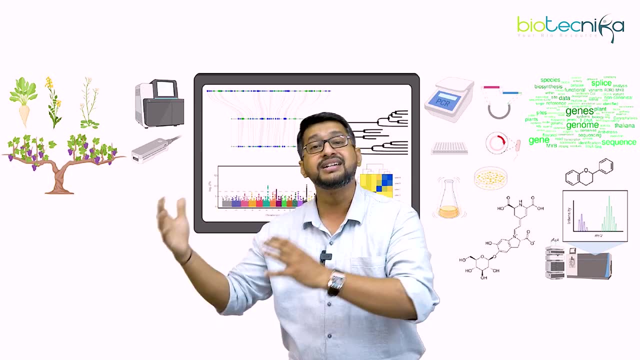 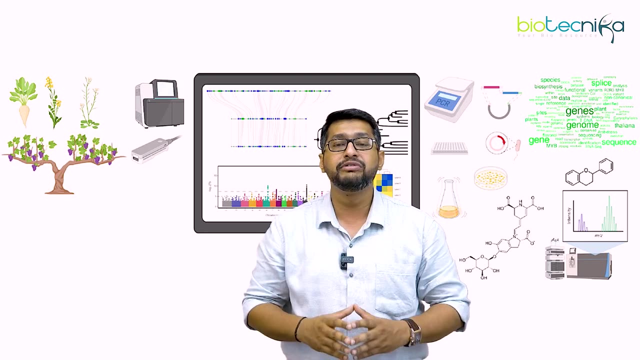 you know, urge people to take up various courses, uh, which can upgrade you, which can make you understand transdisciplinary, interdisciplinary and interdisciplinary sciences, so that you can, you know, start understanding integrative sciences. and this has been possible with various kinds of internship courses and various kinds of certification courses, various kinds of workshops which have been actually.